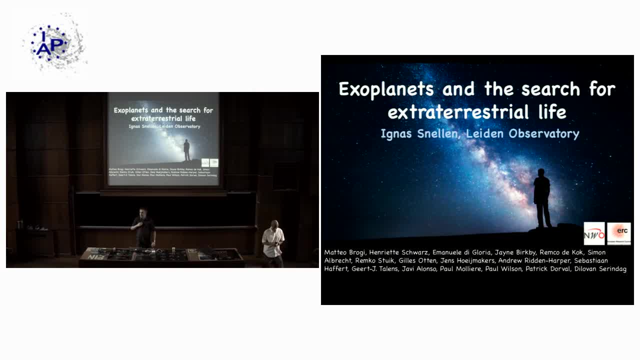 Enya, the floor is yours, Thank you. Thank you, Matt, Is my mic working? Can you all hear me? Yes, Okay, It's very nice to be here. The last time I was here, I was in London. 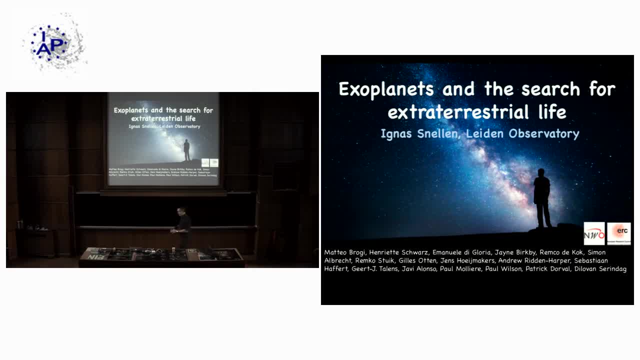 The last time I was in this room was about three years ago, when you had your annual workshop here, And it was so warm that I almost fainted, So I'm very happy it's a much cooler day now. So I'm going to talk about extrasolar planets. 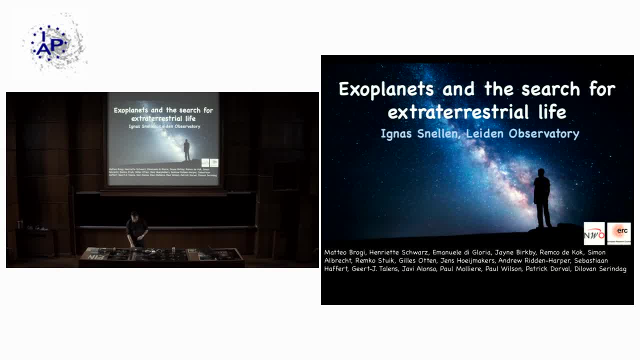 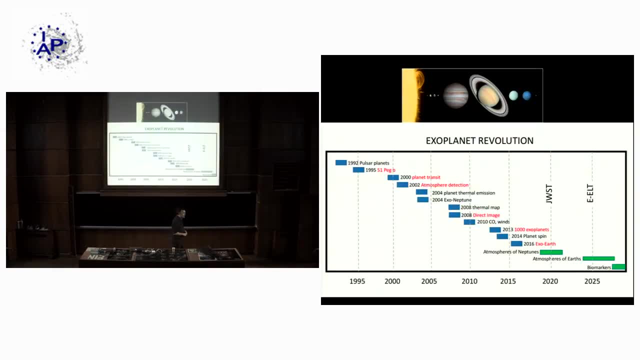 This is a very exciting field And, yeah, when you have been working in this field for a while, like me, then you start to forget that, only about 25 years or so, the only planets that we knew were the planets in our own solar system. 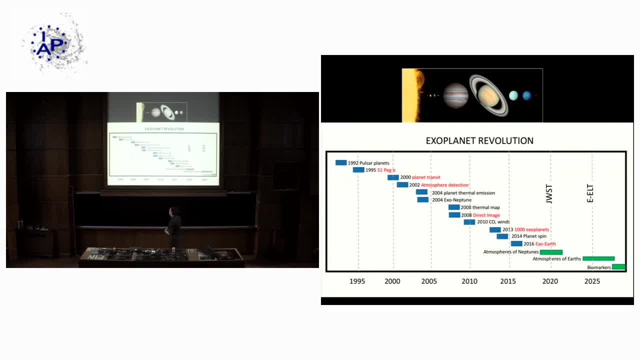 And then in 1992, the first planets in Pulsar systems were actually found. And yeah, the field really started off in 1995 with the first radial velocity planet, 51 Peg B, which orbits a solar-type star. And then, yeah, it's really. you can see, here I sort of indicated the important milestones over the years. 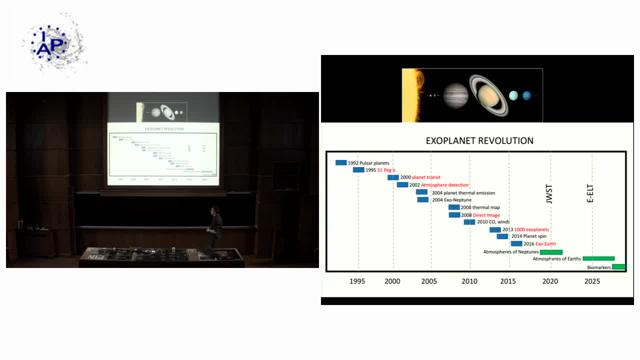 The actual planet, the first planet transits. that led to the first measurement of an actual atmosphere, The first planet thermal emission in 2004.. Then we started to move from hot Jupiter also to smaller planets. The first Neptunes were found. 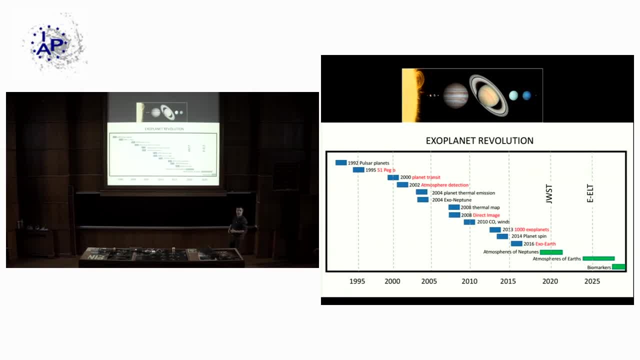 A first thermal map, A direct image, in 2008.. And then we also go to other molecules, molecules and winds. And then in 2013,, about five years ago, we reached a milestone of about 1,000 planets. And then I'll show you a little bit more later. 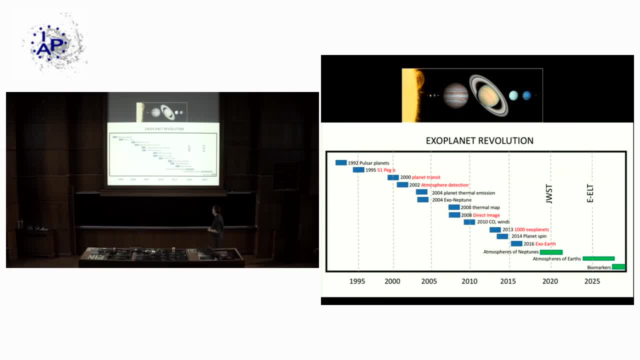 Only less than two years ago now, the first exo-Earth was found. So what is driving this exoplanet, The exoplanet revolution, is not that we are becoming smarter and smarter, but that's because really our instruments are getting better. 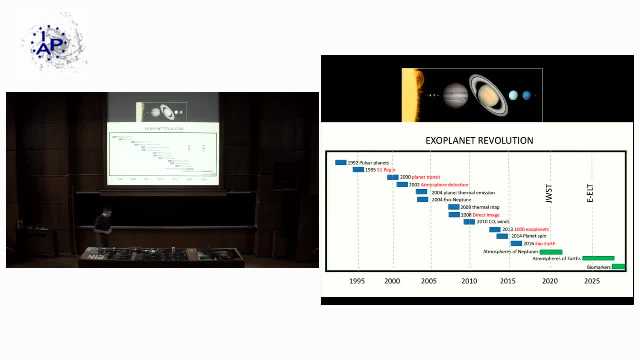 If you only already think about radial velocity measurements, over the course of about 30 years the actual accuracy with which we can do radial velocity measurements has actually increased by about a factor of 1,000. And that is really driving the field And therefore we can also look forward. 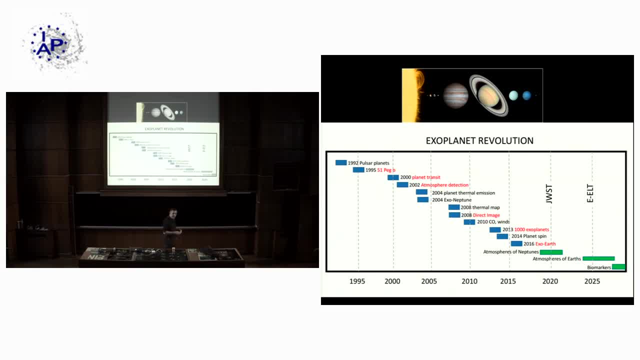 because we sort of know what the next decade is going to give us with respect to new instruments. There are two very important milestones there. There will be the launch of the James Webb, if that will ever happen. This is an old slide, You can see. I still have it there optimistically in 2020.. 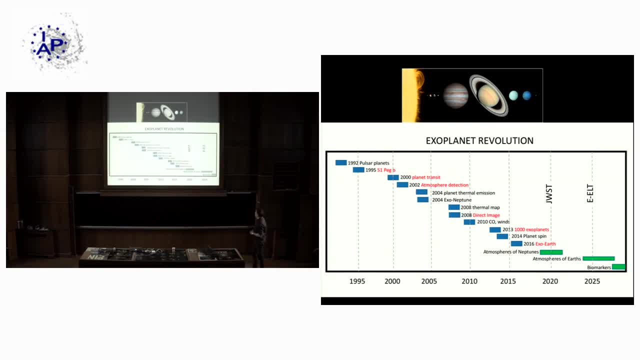 That will of course move a little bit more into the future. And then, very important for my work will be the ELT, which we hope will see first light in about seven years from now, And this really, I think, will move us into the part. 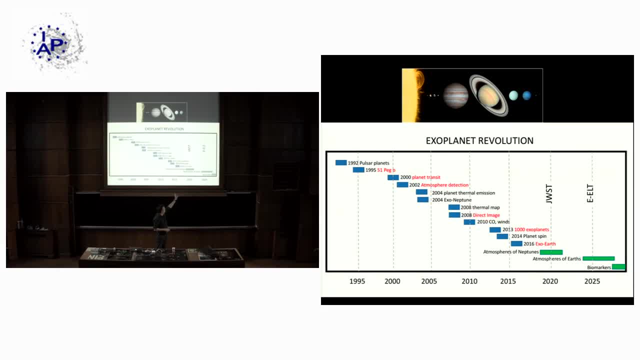 from not only measuring atmospheres of Neptune and atmospheres of Earth, but also into the range where we can start to probe biomarker gases and see whether there are any other planets like the Earth and see whether they actually harbor life. I hear my mobile phone going off. 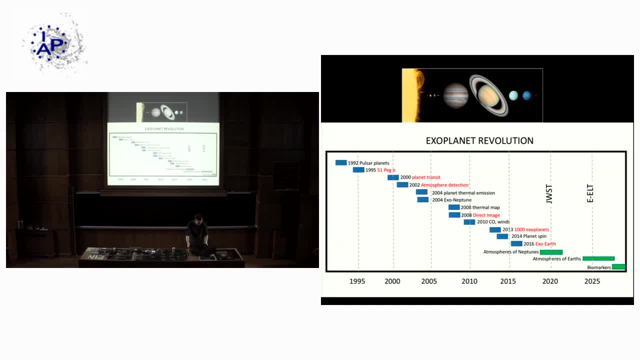 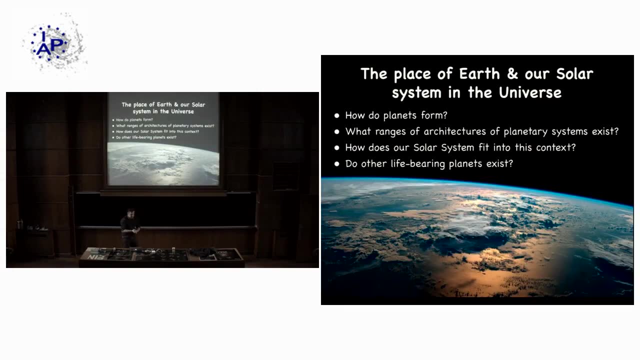 That's probably a good idea to put it out before my mother calls me, or something like that, during the talk. Okay, So let us first go through the main questions of the field. Why do we want to study extrasolar planets? Well, it's all about placing the Earth and our solar system. 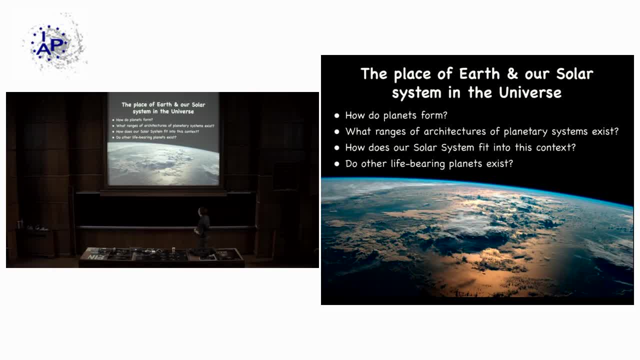 in the context of all planets in the Milky Way and the universe, And we have some general questions. How do planets form? What ranges of architectures of planetary systems exist? Is the solar system typical Or do we really live in some sort of a special place? 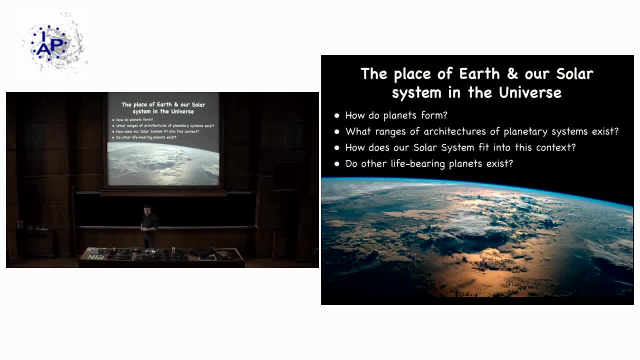 But I really like this final question here Now: do other life-bearing planets exist, Or is the Earth sort of unique in this way? But first, before we go on and talk about exoplanets, it's maybe good just to very briefly, very, very briefly. 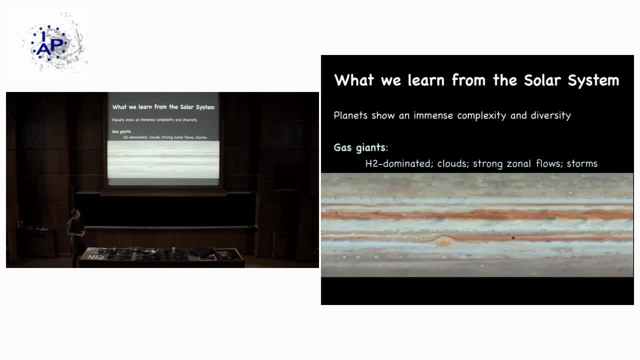 look at the planets, of course, where we know most of, and that are the planets in our own solar system, What we actually already immediately learned from the solar system. looking at the ensemble of planets, that they show an immense complexity and diversity. 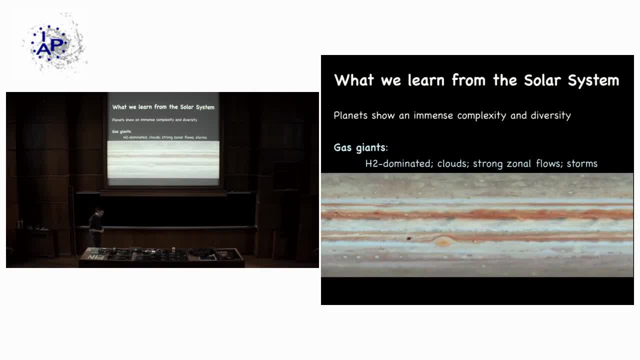 For example, we have the giant, the exo-giant planets. These are molecular hydrogen dominated. They are dominated by clouds, strong zonal flows. They have these storms, like the giant red spots, which has been raging for hundreds of years. 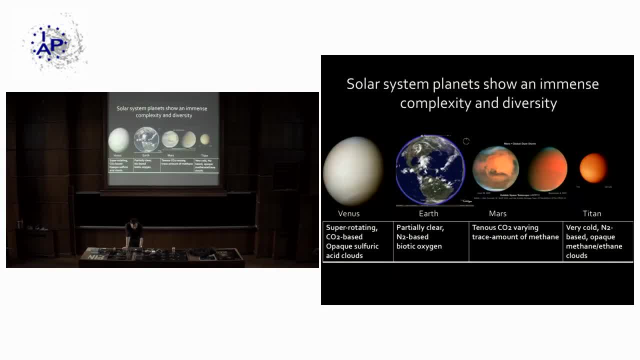 Then we go to the more. when we go to the rocky planets and look at the atmosphere there, we see, yeah, a very clear size of diversity. Now, if we look at the planets and the moon, where we see an atmosphere, we see Venus. 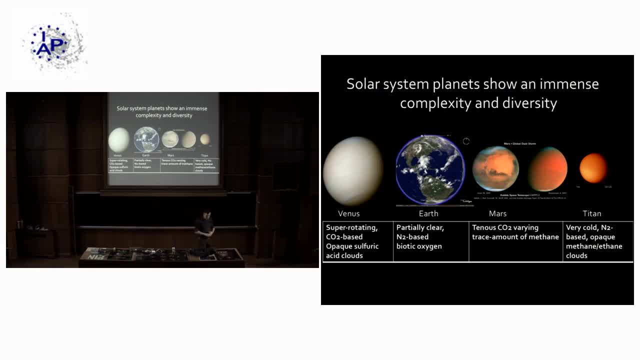 This is a super rotating CO2-based atmosphere. It has these strong, opaque sulfuric acid clouds. Then we move to the Earth. same mass, same radius. It's partially clear. It's nitrogen-based. It has a large fraction of biotic oxygen. 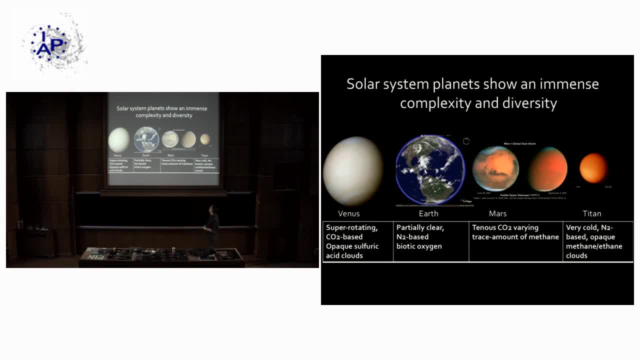 And then when we go to Mars, that has again a CO2 atmosphere Very thin. It has, for example, a trace amount of methane of which we don't know the actual origin yet. And then when we look at Saturn's moon, Titan, 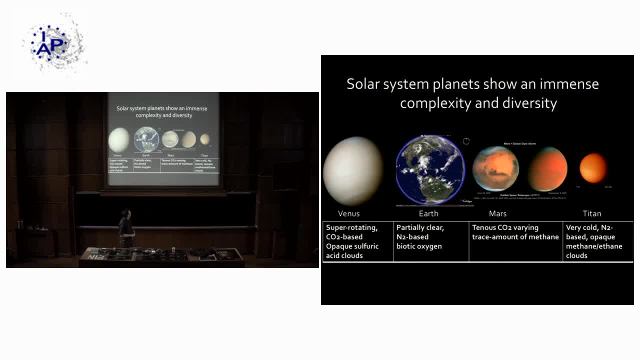 there we again see it is a nitrogen-based, where we see opaque methane and ethane clouds, And they have also not a water cycle but a cycle of methane and ethane on this moon. So I think it will be very difficult if we would only have the solar system. 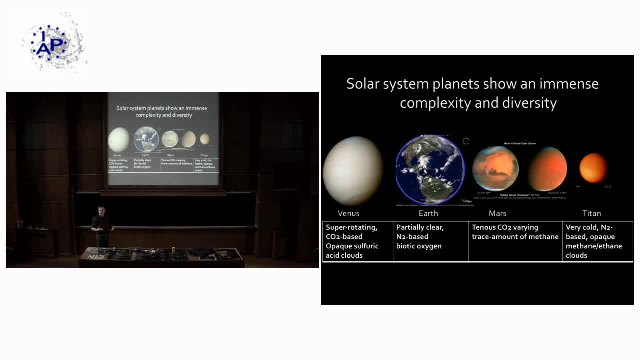 and come up with a general theory of planets, identify different families and see now what is the origin of these different atmospheres. Of course you can make up theories why these differences are there, but how do we know that these theories are right? 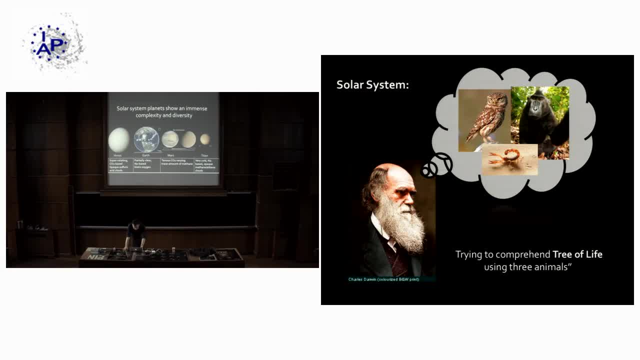 And I'd like to make. I'll show an example. The way I see this. it's like one of my heroes is Charles Darwin, And it would be the same if Darwin had to find out the actual trees, the tree of life. 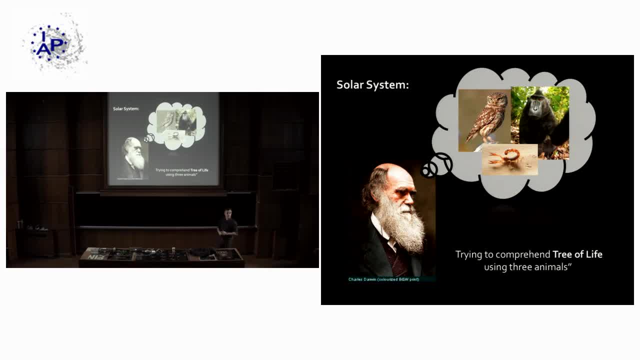 when he would only have access to three, three or four animals. Now, how do I link this monkey to this owl and to this scorpion? I think with just three animals or three species, this is not possible, And he also recognized this. 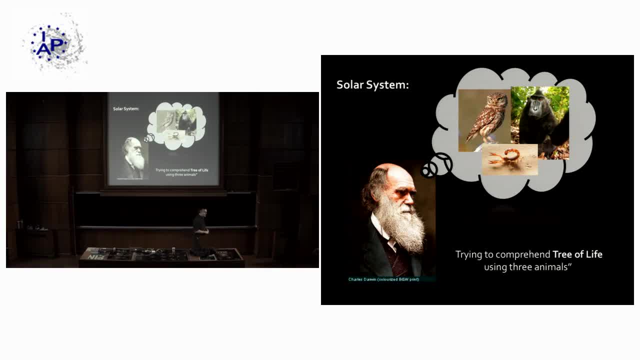 so he went on this epic voyage on the Beagle, went to distant shores and islands to find out about all these different families of plants and actual animals, And in this way he came back with his great theory of evolution And I see the exoplanet science also a bit like this voyage. 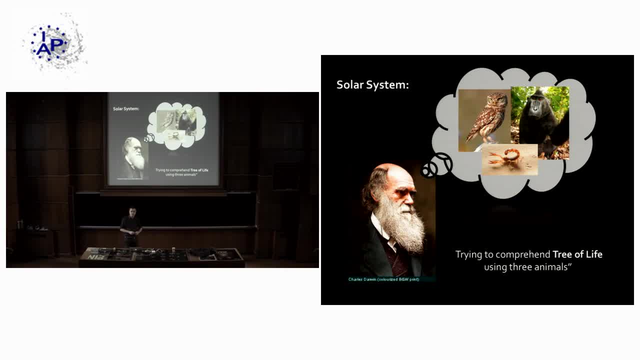 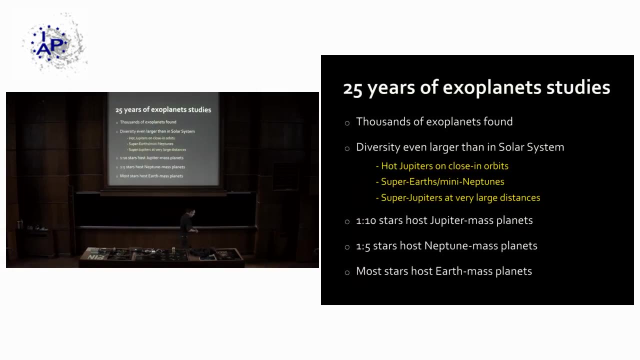 It will be very difficult. it will be very hard to study exoplanets, but we really need it to actually understand the general formation and evolution of planet systems. So we have now about 25 years of exoplanet studies. So what have we learned so far? 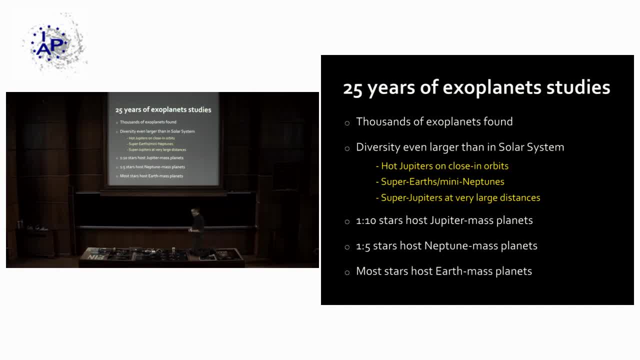 Well, typically about you know, more than a thousand exoplanets have been found. They are very common And immediately we see that the actual diversity is even larger than we see in our own solar system. We have, for example, the hot Jupiters. gas giant planets in very short orbits? We have no idea. Well, we are quite sure that they haven't formed at such a short orbital time, so they have to have formed much further away from the exostar and in some way have migrated inwards. 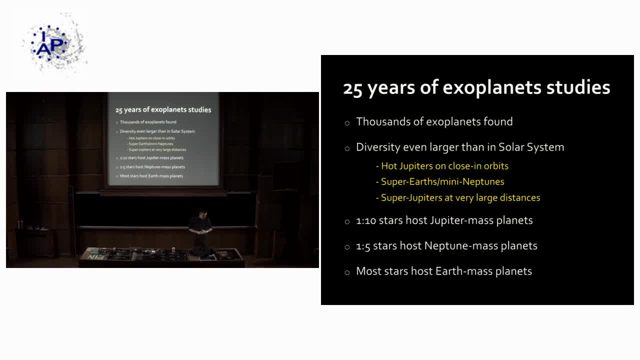 Then we have this typical class of super-Earths or mini-Neptunes, also a type of planet very common but it's not seen in our own solar system. And then we have these super-Jupiters, these very massive gas giant planets. 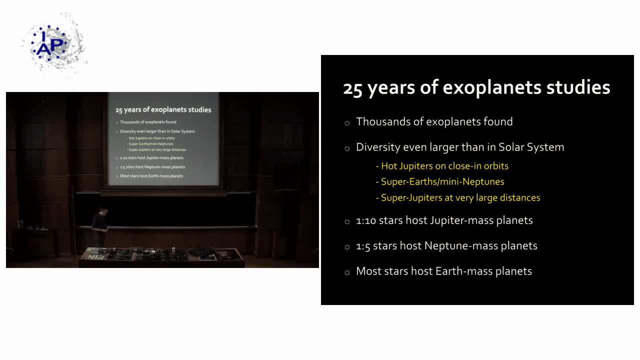 that are at very large orbits, at very large optical distances, orbital distances up to 100 AU or even further, And also for those it's not clear how such planets could actually form. Now we typically see that for solar-type stars, about 1 in 10 stars host a Jupiter-Mars planet. 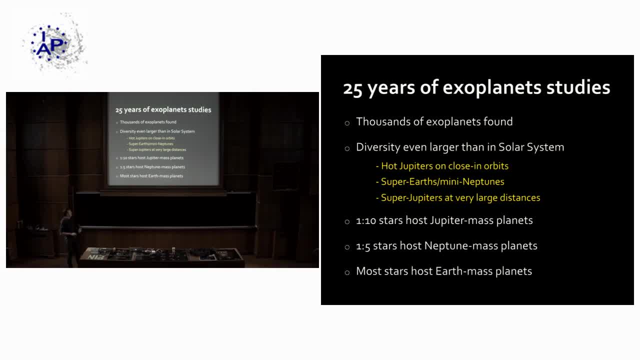 so maybe that fraction is actually a little bit higher. We have about 1 in 5 stars host a Neptune-Mars planet. Most stars host an Earth-Mars planet. So I'm not talking here about Earth-like planets. No, I'm not talking about planets that have oceans and trees. 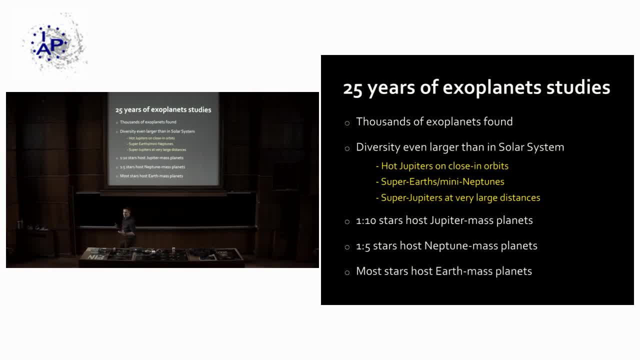 and things like that. It's just a simple parameter that the masses of the planets are about that of the Earth, but they could be at any orbit. Now, what I think it is, of course, in the end, at least with my research, we hope to zoom in. 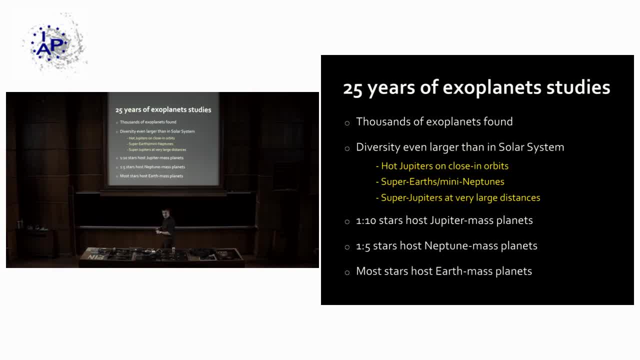 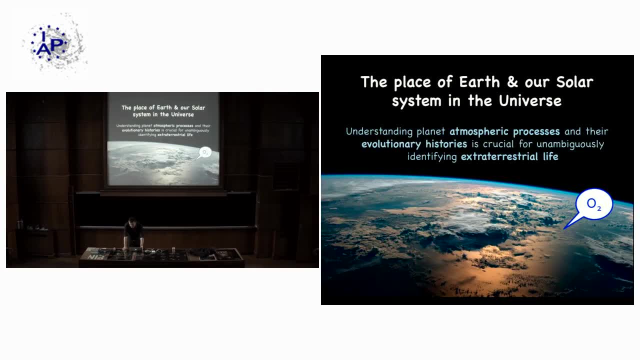 on trying to identify planets where life is possible and maybe see whether there is actually life on such a planet. But I also want to say that to be able to do this, we must have a much broader understanding of planets, their atmosphere, how they form. 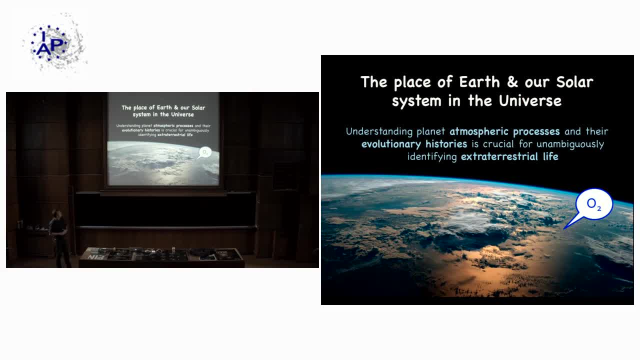 and how they actually evolve. Only by understanding the atmospheric processes and their evolutionary history it will, in the end, be possible to actually unambiguously identify extraterrestrial life, And what I mean to say by that is at some point, I hope, in the next decade. 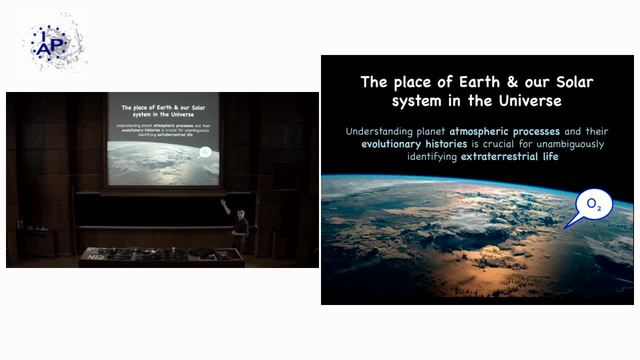 we will identify planets where we see, for example, oxygen And we know on the Earth oxygen is due to life. But yeah, that doesn't mean that on another planet this oxygen is actually due to life. We can only find out after we really have understood. 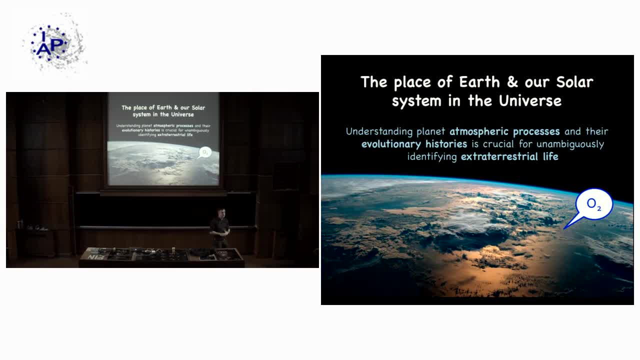 all the atmospheric processes that can happen in such a planet before we can really identify it to be due to biological activity. And this will be a very difficult and long path where many different disciplines from biology, atmospheric physics, geophysics have to come and work on these type of problems. 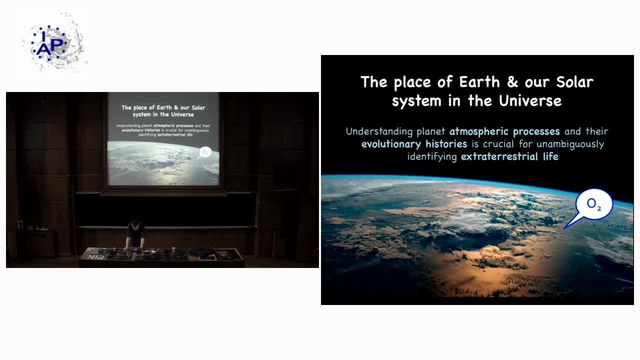 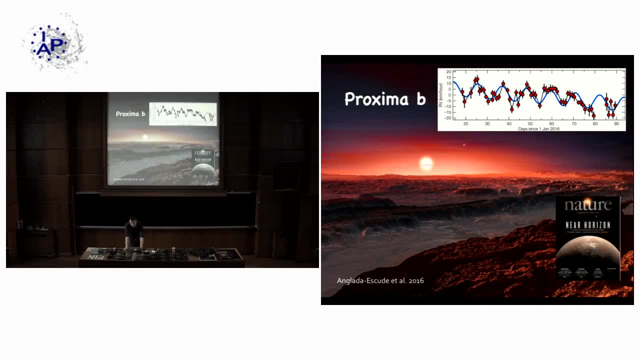 Okay, the great news is that, also in recent years, the progress has been quite amazing. We now have started. we now have a sample of planets about the size or mass of the Earth that seem to be in the habitable zone of the star. 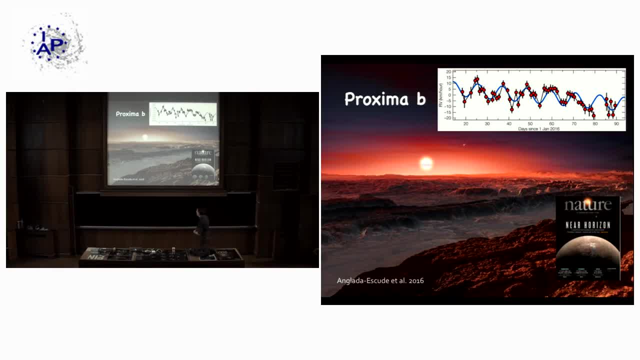 meaning that possibly liquid water could be present at their surface. First of all, there's, of course, Proxima b, found about one and a half years ago with the HARPS spectrograph. It's in an orbit of about 11 days. 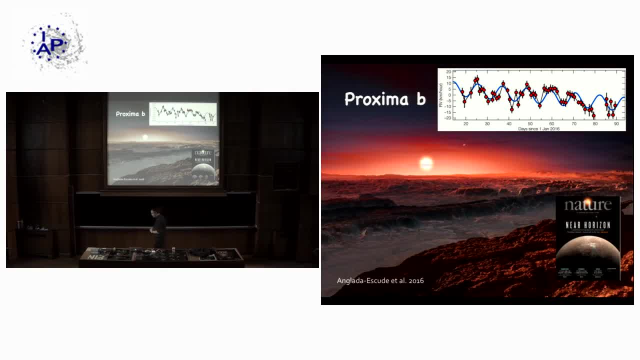 but because Proxima b is such a small and faint star, an 11-day orbit means that it actually receives about 30% less energy from its star than the actual Earth does, but that's still more. that's still about 60% more. 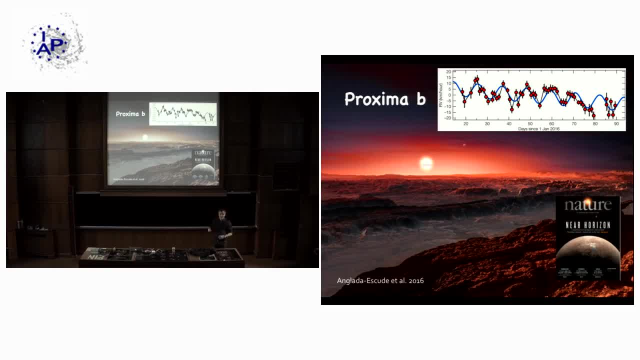 than actually Mars does, So it should have a climate somewhere in between that of Mars and the Earth. Now, of course, we don't know whether life could be, could actually be present on such a planet, because the actual star is not so nice. 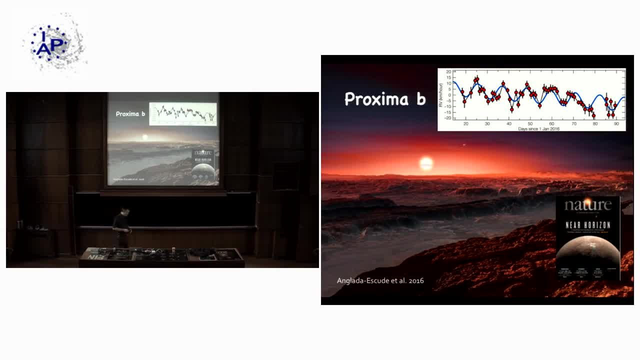 This Proxima sends out flares. There are all kinds of problems with the actual history of such a star that in the early history of Proxima it should also be radiate a lot more energy and therefore it should have been a lot hotter. 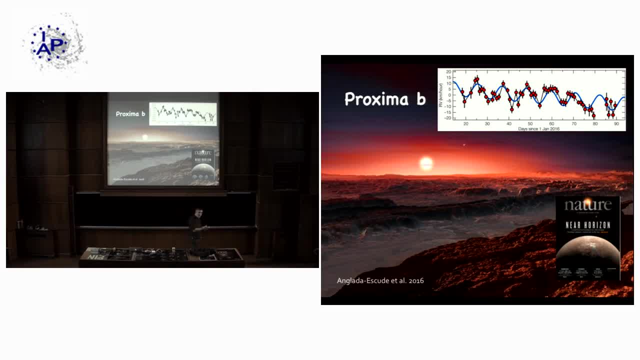 The actual planets are locked, so there's always one day side and one night side on such a planet. so it's not clear whether life could actually exist on Proxima b, but still, you know this will be. this is such a great sample to start looking. 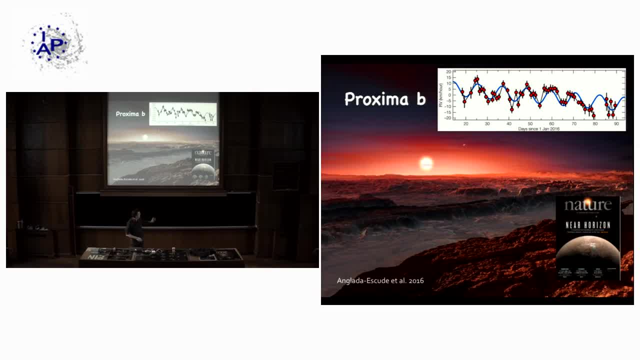 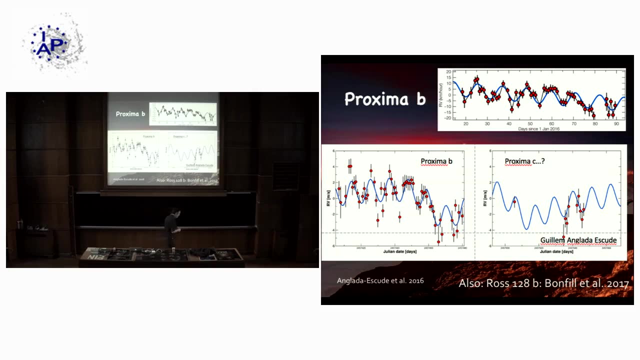 and see what kind of climates are, what climate is actually present on this planet. that, yeah, we can really start doing this in the next decade. It turns out that these rocky planets are very common around nearby M dwarfs. This, actually, this is very nice work on Proxima b. 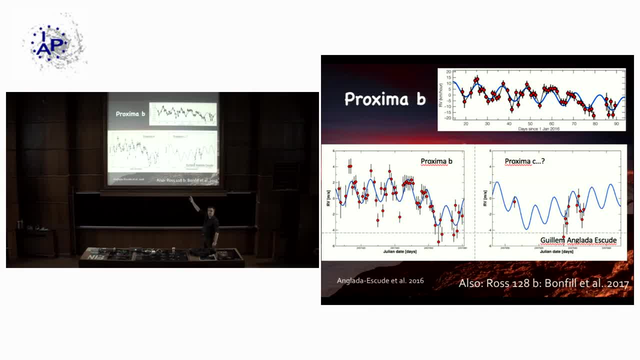 They have a nice website- It's the pale red dot website where you can see live the radio velocity points coming, coming actually in, and they have another. a half year ago or so they had another session on Proxima and there may also be an actual evidence. 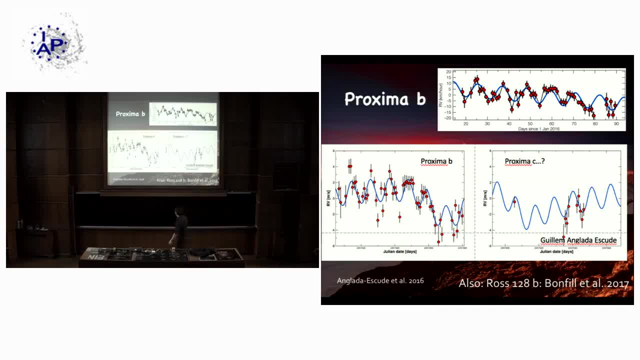 for a second planet, so there could be a Proxima c. There's also some other work, that of the nearby star Ross 128, which also shows to have a rocky planet. Now, that's all radio velocity work. That's also the transit work. 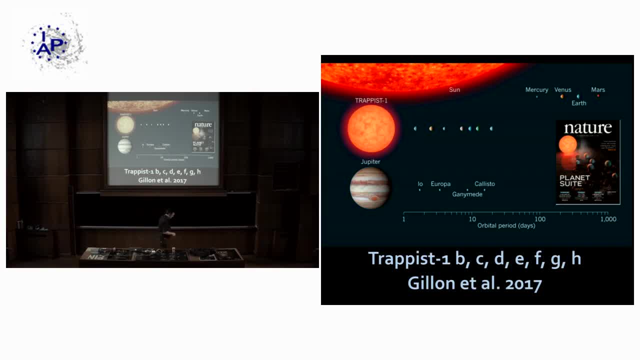 This is also some work that you get really jealous of when you see it. This is, of course, the TRAPPIST-1.. Now, this team really went out starting a couple of years ago. what if the lowest mass stars? so we're talking about an M8. 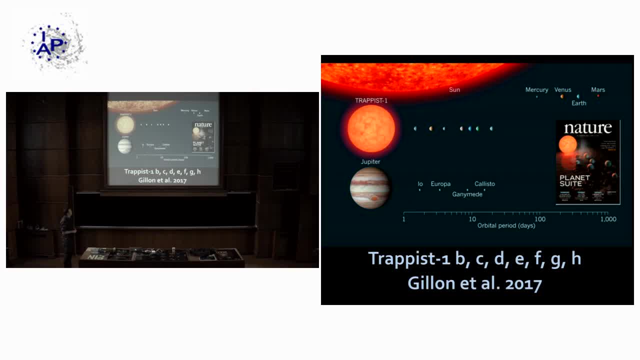 or even high mass brown dwarf stars do have planets, right. Shouldn't it be much easier to actually see them using transits? So they started to monitor about 50 stars and already within a couple of months they found TRAPPIST-1 b. 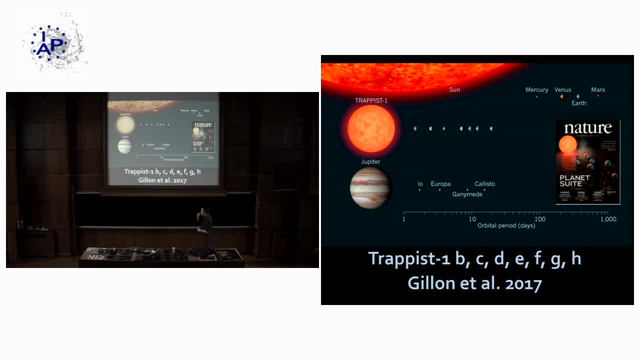 so they found the first planet and I think they also found TRAPPIST-1 c, and then they got a lot of spitzer time. I think they got 30 or 40 days of spitzer time where they monitored the whole system. 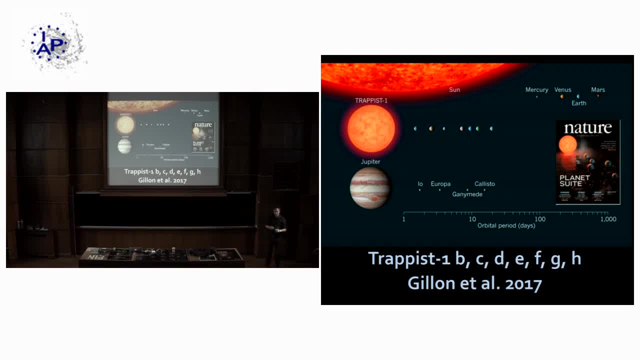 because next to TRAPPIST-1 b and c they found a single transit and they thought: hey, so there must be a third planet there. So they monitored for a month or so and they found seven planets, all very nicely aligned in. 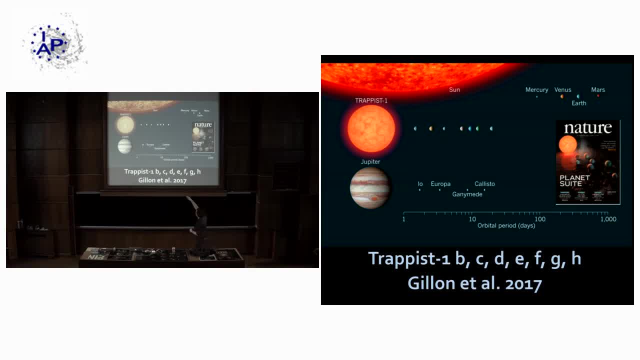 yeah, you can see the exo-orbital space. you can see the exo-orbital periods here. It's ranging from 1.5 days to about 20 days. They're all about the size of the Earth and if you think about how much energy. 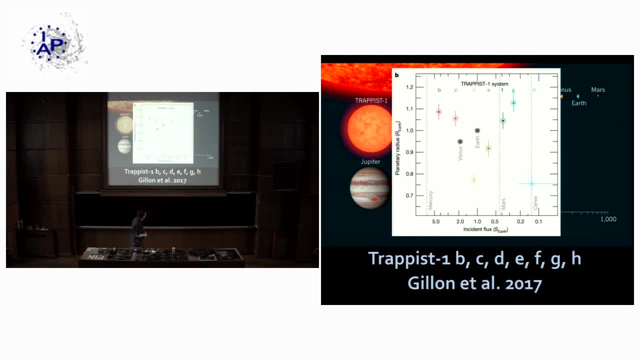 they receive from that star. this is the incident flux here on the horizontal axis. they're about three or so, three of these planets that are in the so-called habitable zone that could well receive so much energy and could have liquid water on their surface. 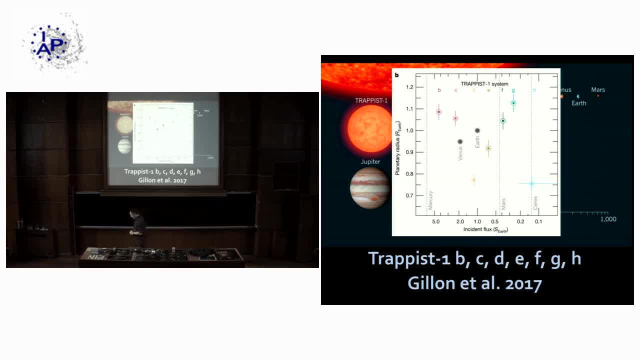 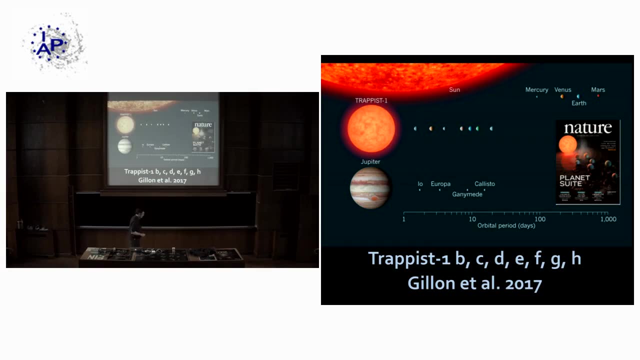 So this is all really very exciting and again, hopefully in the next decade or so, we can really probe the atmospheres of these planets and see, yeah, what they are actually made of. Also, what I really like about this system is that they found it only out of. 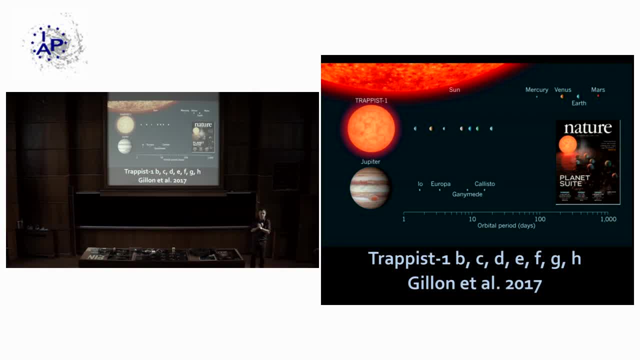 a very small sample, meaning that either they are very lucky or this kind of planet systems are very, very common, because you have to have the right orientation to see these planets transits. There is only about a 1 in 40 or so chance. 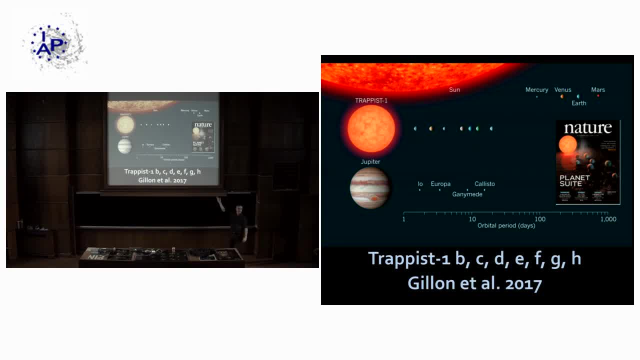 so if you would have a random orientation and they only found it out of a sample of 50 or so stars. So that basically tells you that these planets are very common and we will soon learn that from this group who is observing now a larger sample. 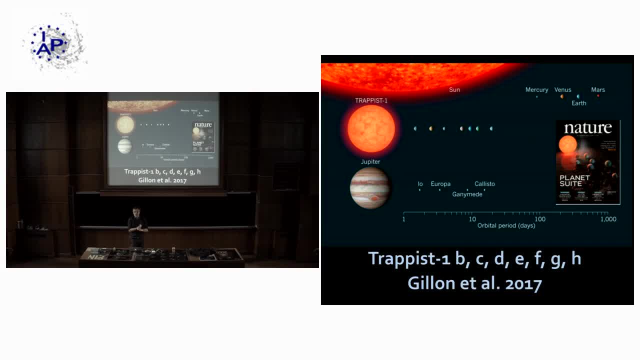 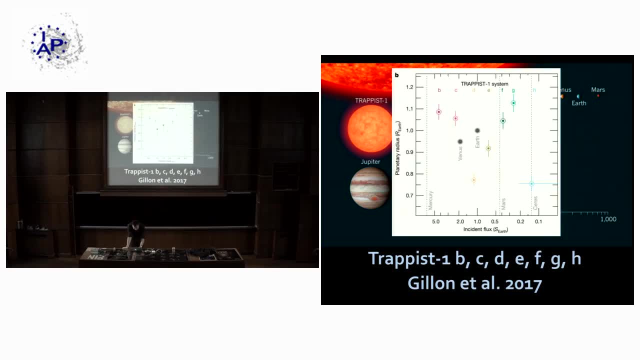 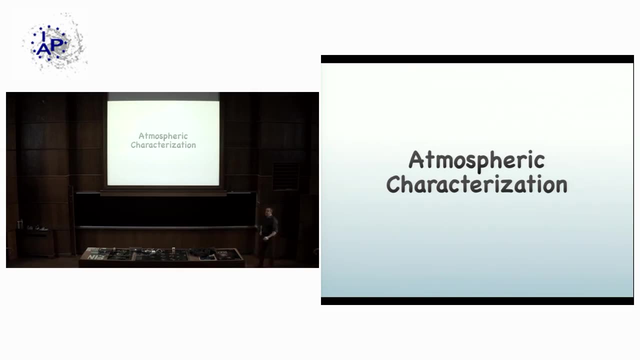 And that these planets are common. we know that also from Proxima B, because our nearest star has actually a similar planet as these. Now, this is all so far, all about finding planets. My work is more about trying to learn about the atmospheres. 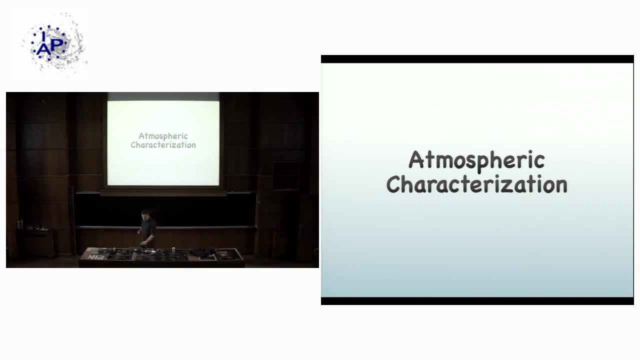 and there the game is somewhat different, in the sense that I've told you that thousands of planets have been found, but for most of these, not a single photon has been identified coming from the planet themselves. If you do radio velocity methods work, even if you do transit work, 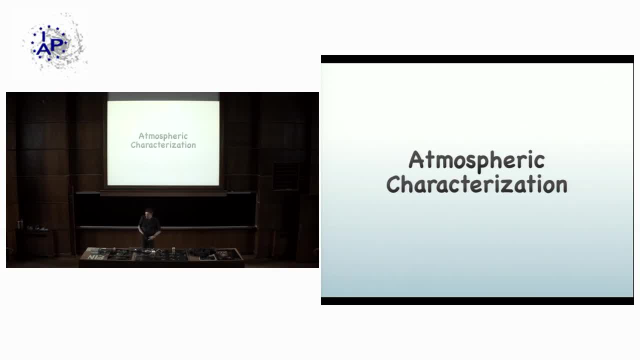 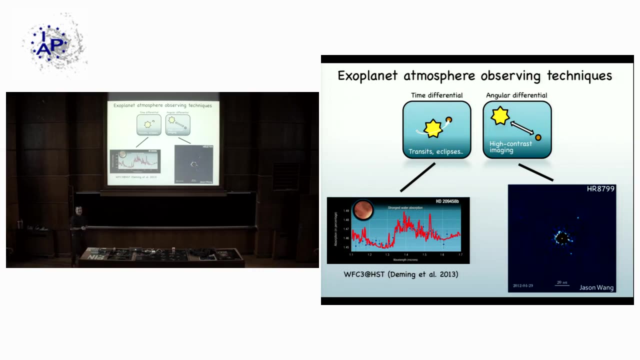 it's not that you see photons from the planet. If you do atmospheric work, you no longer cannot do that. You have to separate light out which is coming from the star and coming from the planet, And there are basically two families of methods to actually do this. 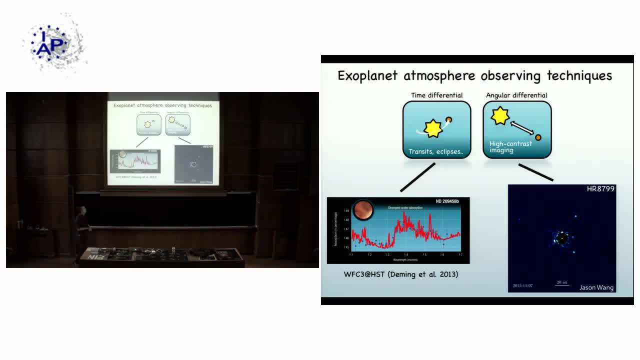 I call them time differences, a differential method and an angular differential method. You could also simply say one is sort of the actual transit method and the other one is the direct imaging method. So the direct imaging method: you spatially separate the star light. 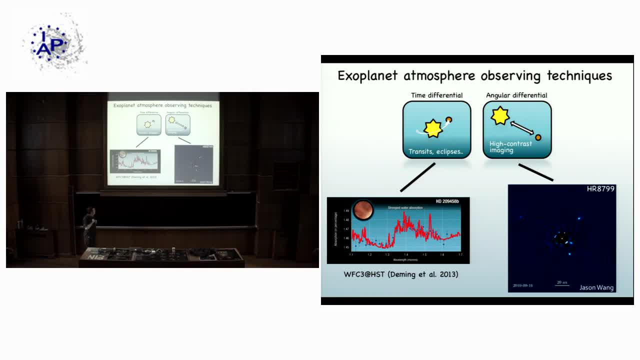 from the planet And, Yeah, it's still working. This is a very nice example. It's, at this point, still very difficult to get the contrast, because the expected contrast between the star and the planet are very high, but not so much for the very young systems. 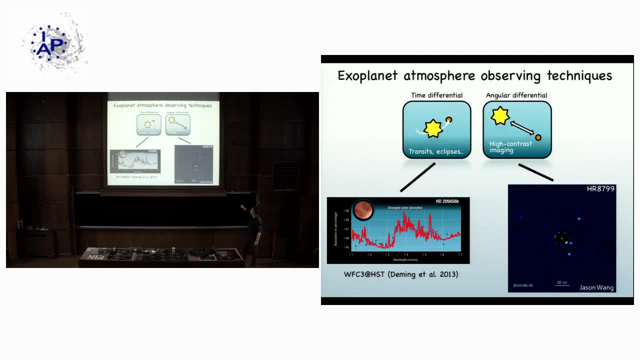 so typically 10 million years old. This is an example. This is a young, A star: HR 8799.. And you really have a family portrait of four giant planets here, And it's nice now, over the course of several years, 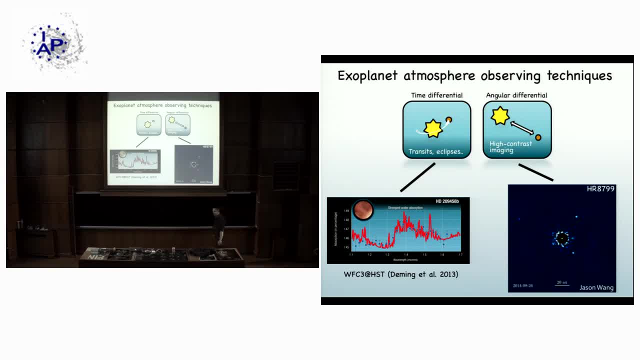 you really see the exoplanet move around the star. So that's one way. That is the angular differential method, The time differential. we are talking about transits and eclipses and phase curves And that makes What happens. there is that. 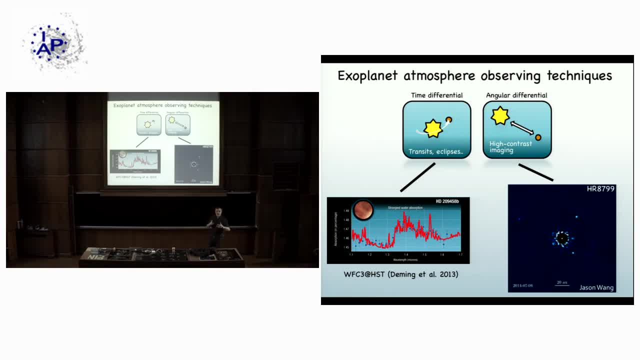 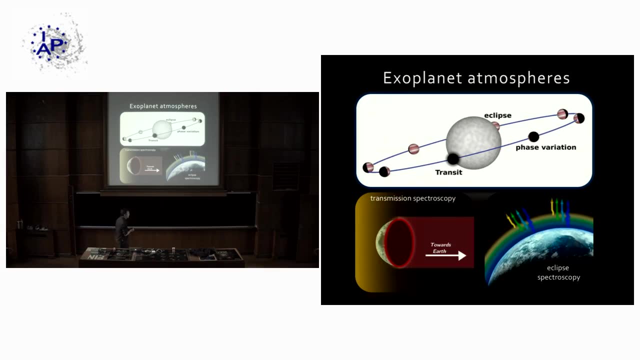 as a function of time, we see the planet light differently. So, for example, only during the actual transit you see the actual star light filtering through the atmosphere of the planet. And I have a slide here. Is there a pointer which I can use? 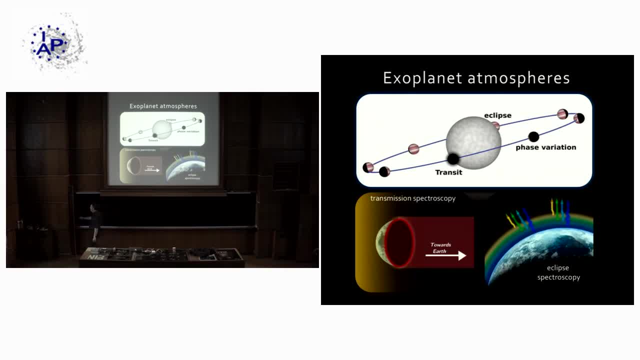 Oh, here it is. I see a big stick. I see a big stick. It's all right. Yeah, it's physical, I like it, It's good. So what happens when the planet orbits the actual star? at the moment, the planet moves in front of the star. 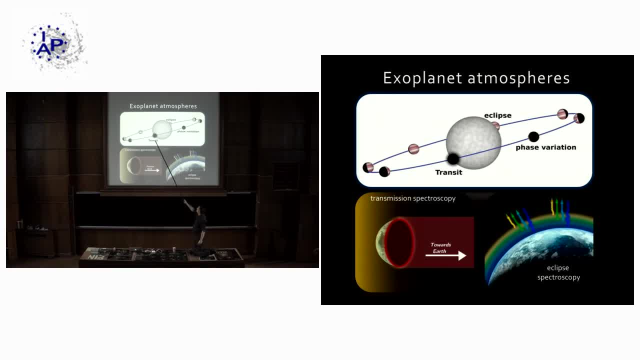 of course some star light is blocked by the planet, but also some light filters through the atmosphere and leaves an imprint of atomic or molecular absorption or scattering processes. Then half an orbit later, the planet is actually eclipsed. That is So for a moment. 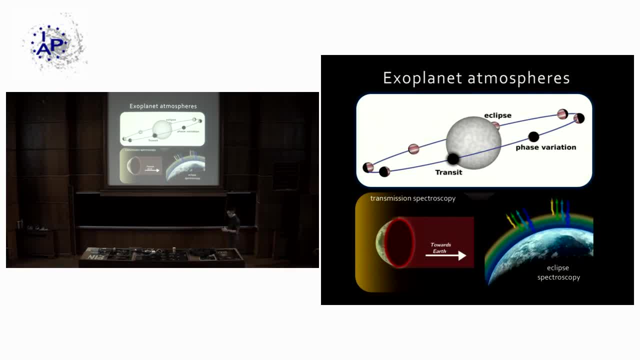 we don't see the exoplanet light, So the light missing, that could be reflected light, or the cold could be direct thermal emission from the planet. We can actually measure in that way. And then what can happen is if we monitor a system, 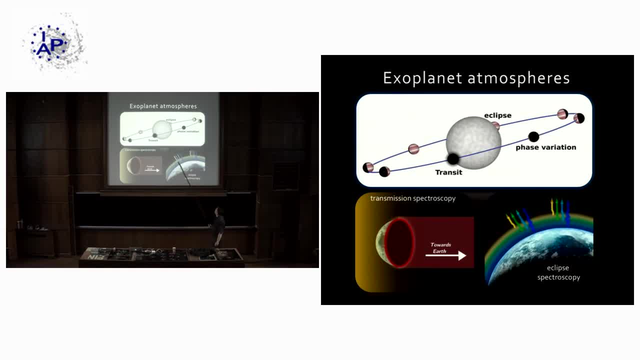 then we can really see the phase variations, meaning that near the transit we look at the cool night side of the planet and then near the eclipse we see generally the hotter day side. So that can tell us something about the temperature structure around the planet. 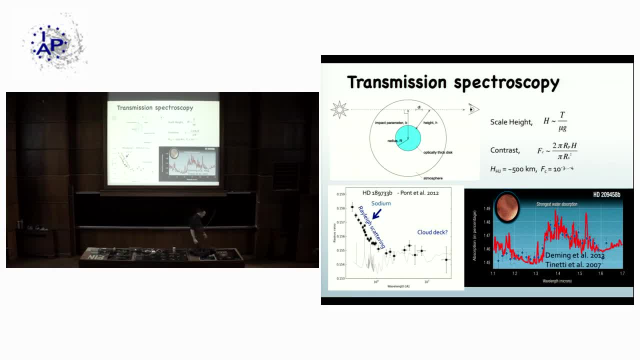 Just to give you a short intro of what we actually measure when we take a transit spectra, it's basically the effective size of of the exoplanet moving in front of the star. So if we observe it at a certain wavelength where the atmosphere absorbs, 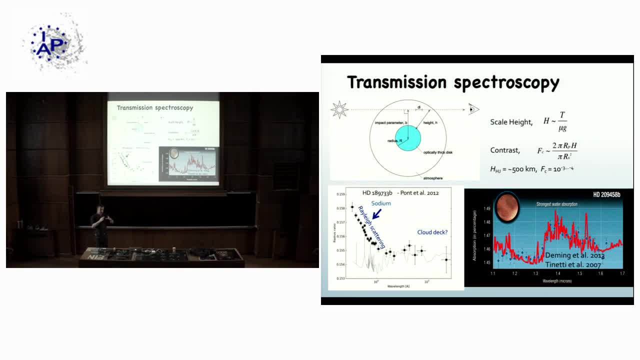 then the absorption of the atmosphere makes this planet size a little bit larger And therefore it seems that the exotransit at that wavelength is actually a bit deeper. So when we see, when we plot the transit, the exotransit spectrum, like here: 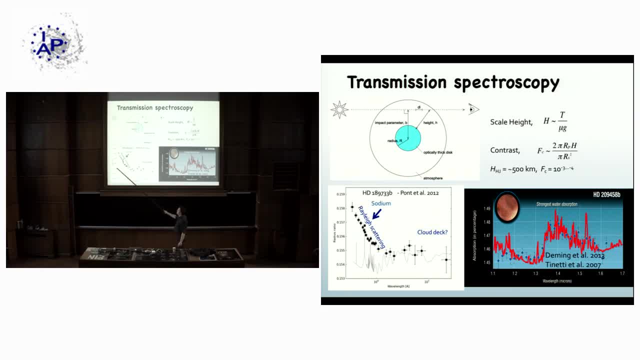 we see here the radius ratio with what we actually measure is the transit depth, So the transit depth as function of wavelength. And this is, there are two planets with which we can do this very well, That's two hot Jupiters. 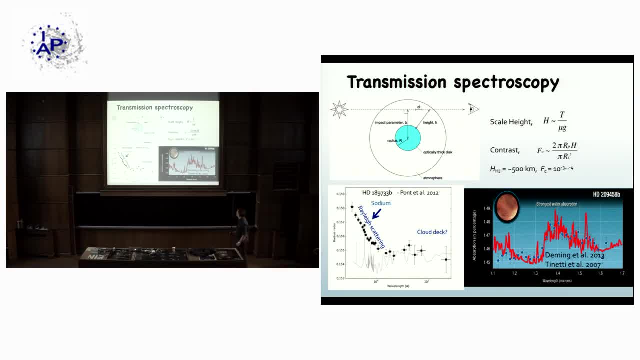 HD 189 and HD 209458. So you see both examples here. So this is a transit spectrum very famous where we see in the UV optical that the effective radius of the planet is significantly larger And we think that this is due to Rayleigh scattering. 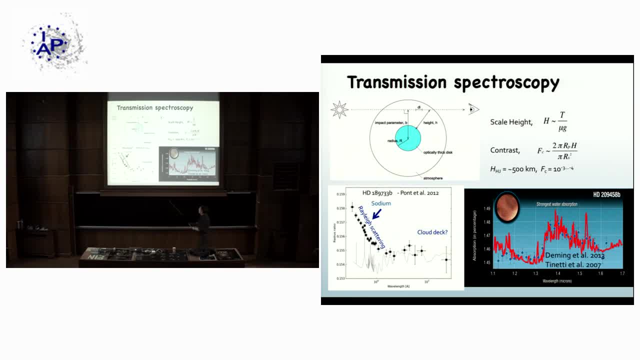 of haze particles high up in the atmosphere And then it sort of flattens out. Now these observations: they don't really show any other absorption features, But there may be a cloud deck, but there's also now some exomolecular features are seen there. 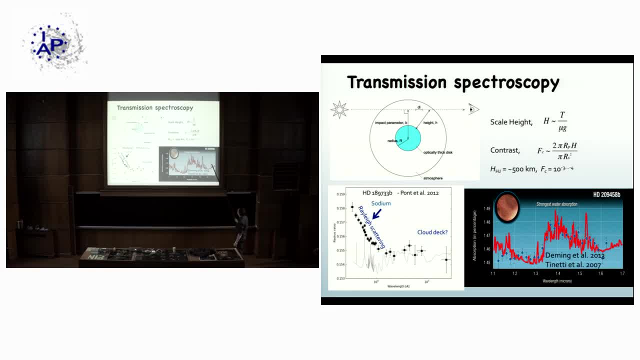 For example, water, And this is a nice example of HD 209.. The blue dots is the data here. So again, this now says absorption, But this is again. this is actually planet radius, or it is transit depth, And you see very nicely. 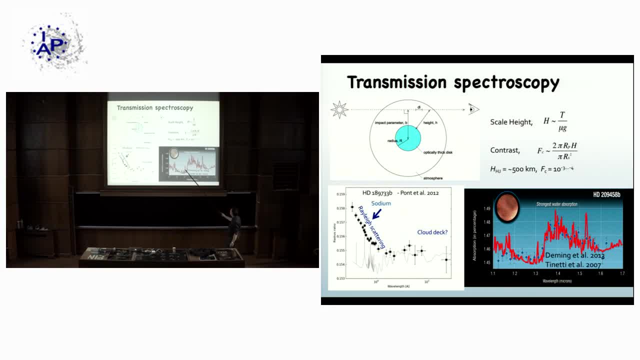 so there's no variation in transit depth here, And then around 1.35 micron, it shoots up. the planet is larger And that is because of extra absorption in the atmosphere due to water. In this way, water is seen also now. 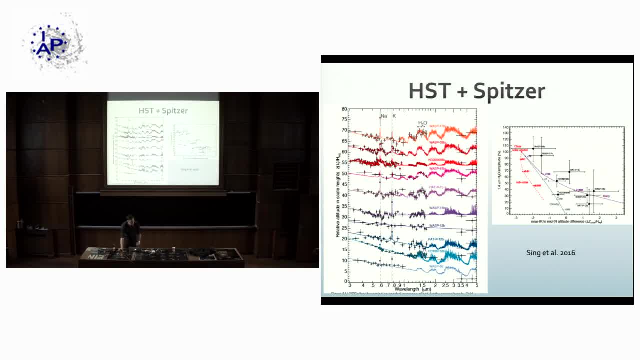 for an all ensemble of planets at about 12 or so hotspots, and also hot Jupiters. This is seen both the Rayleigh scattering slope and the actual water absorption. And, what is very nice, this is David Singh's work, who used to be here in Paris. 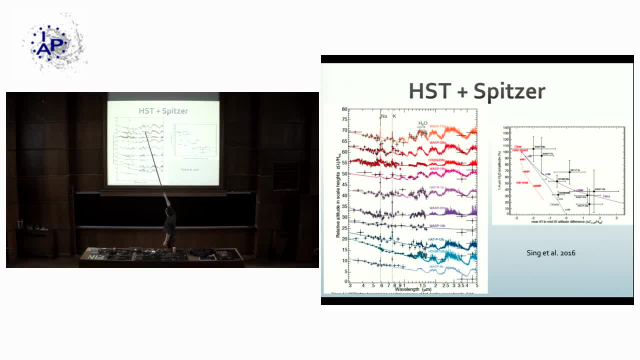 I think, where what they observe is that when you don't hardly see any Rayleigh scattering slope, there seems to be a strong water feature, And if you have a strong Rayleigh scattering slope, the water feature is much more muted. You can see that here. 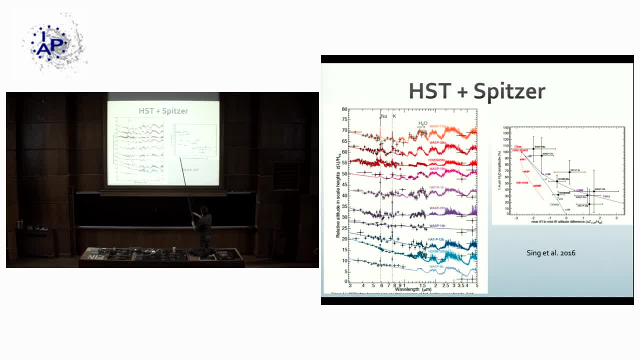 this is sort of the Rayleigh scattering, a measure for the Rayleigh scattering slope, the prominence of the Rayleigh scattering slope and this is the water absorption. And the idea here is- and I think now we're really starting to learn some physics- 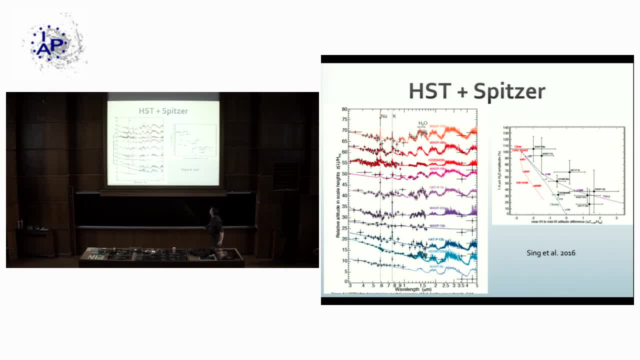 in the atmosphere of these hot Jupiters is that when you have a strong Rayleigh scattering slope, that means there are hazes high up in the atmosphere that mute the actual water signature. So yeah, and you have strong hazes. 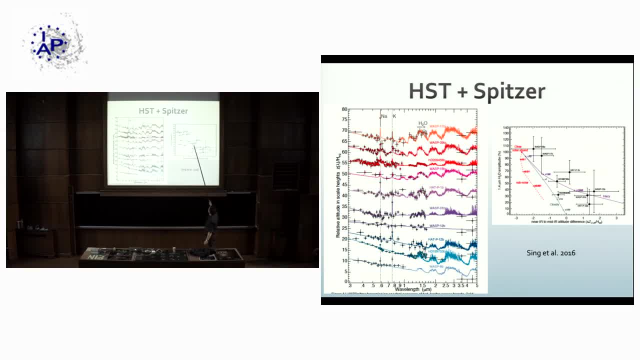 you don't see the actual water If the atmosphere is clear- sorry, if you have strong hazes- you don't see the water. If the atmosphere is clear, you see a strong water feature. So the variation is probably not caused by different volume mixing ratios. 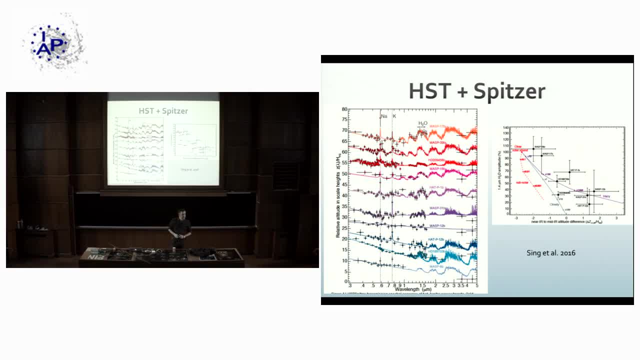 of water in these planets. These planets are probably all very, very similar, but it's just. one has hazes and the other one don't. Still, we don't know why some planets have hazes and others don't, but that's a whole new. question. Now, several groups have started to move away from hot Jupiters and going to cooler planets. This is easiest done when these planets orbit small stars, and that's because the actual ratio between planets and stars is then significantly larger. This is an example of GJ 1214,. 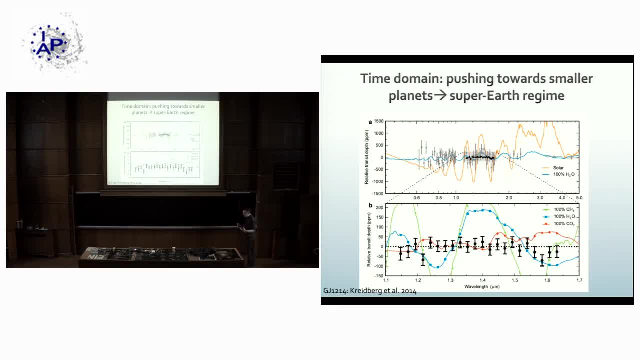 a sort of a super Earth or a mini Neptune, And the nice thing about these planets is that this is basically a new class of planets and we can, basically we can solve for the mass-radius relation in two ways. Either these are volatile-rich planets. 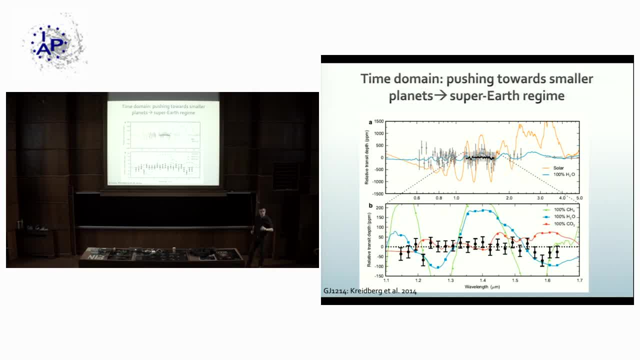 so they may be very water-rich, or these may have a rocky core with a hydrogen envelope. Now, how could you measure the difference between these two? How could we find out the difference? Well, if the atmosphere is water dominated, then the scale height. 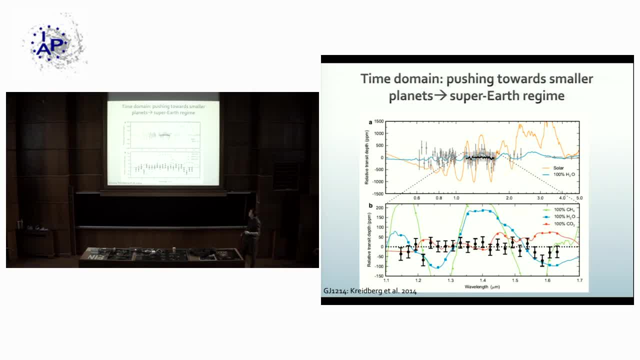 of the atmosphere is much smaller, You would expect much muted signals, transit signals, while if it was a hydrogen atmosphere, you would expect very strong signals, And that is what you see here. This is what you expect: the variations from water in a hydrogen atmosphere. 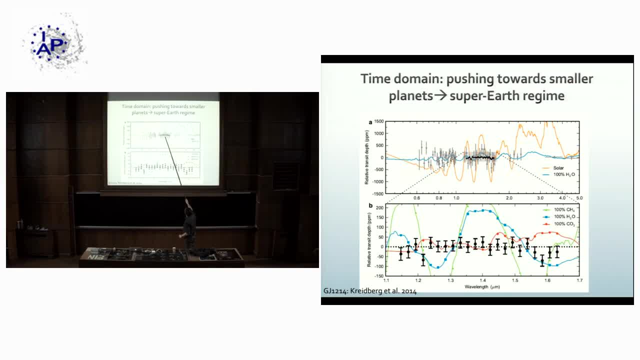 and this is for a water-dominated atmosphere, And when you zoom in, you see actually that the data is very flat, You don't see anything, And so, even for a completely water-dominated atmosphere, you would expect a much stronger signal than is seen. 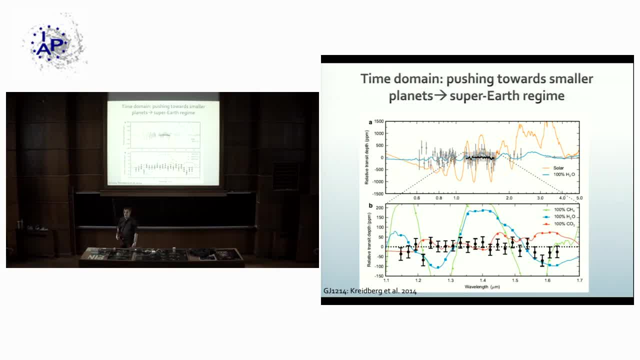 And the general idea here is that there are actually clouds, clouds that are very strongly muting the actual atmosphere. So this is one of the challenges that we will face in the future of this kind of atmospheric work. I don't have time for this. 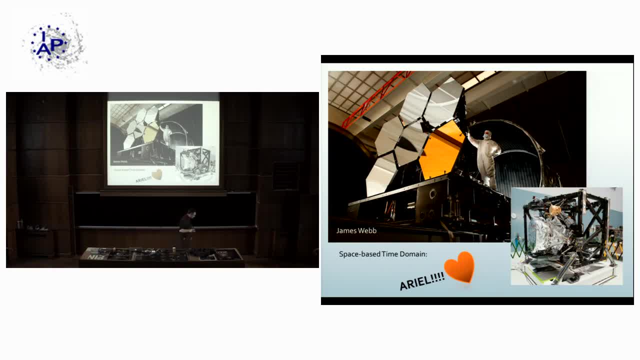 I want to say a little bit about the future. This type of work works very well from space. There is, of course, the James Webb is going to be launched soon, but also a very exciting Ariel. I understand the IP has a very strong role. 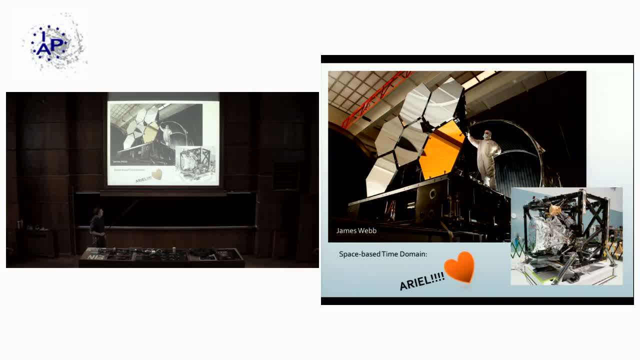 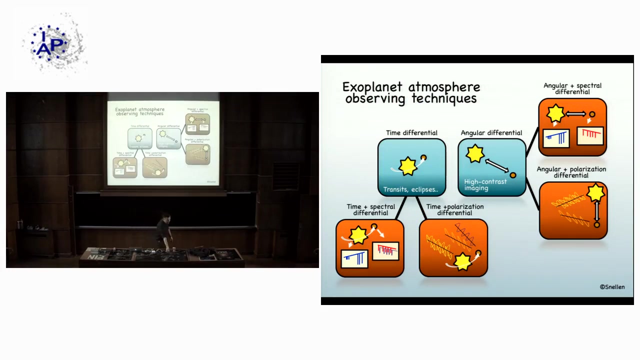 in this, in this mission, And we're all very happy that it got selected by by ESA, And it will really observe a very large sample of these warmer, warmer objects. Okay, now I'm about halfway in my talk, So I want now to talk about our own work. 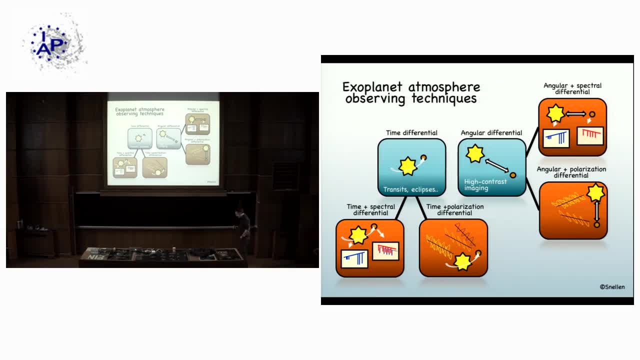 This was a general overview of the field And in my group we really focus on trying to do these atmospheric studies from the ground And what we have found out is that both the transit method so the time differential methods, as the angular differential methods, 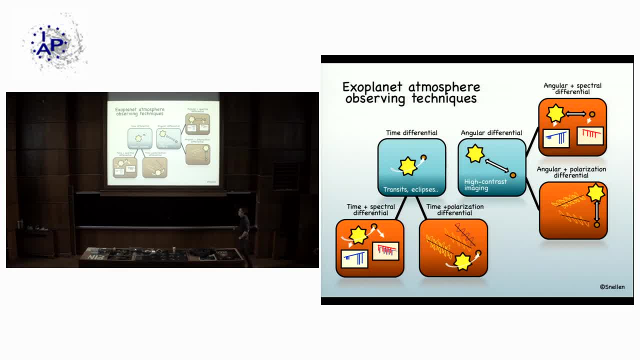 work very well if you combine them with high dispersion spectral observation And the idea behind that. so by the time difference between the signal from the planet and the star, you can already separate out the planet from the star. But what helps if you then get 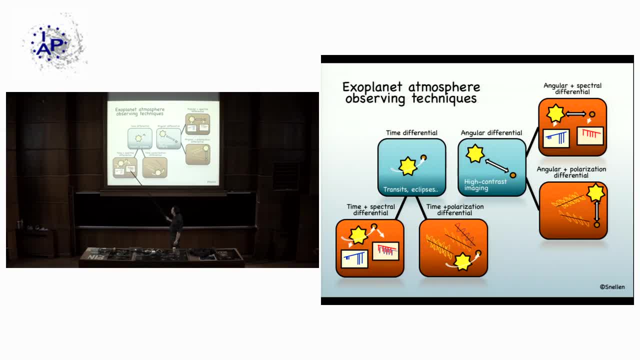 an extra measure, and that is the spectrum, because you also expect the spectral lines of the planet to be very different from the star. So in that way you can actually have an extra measure to separate out the light coming from the star and from the planets. 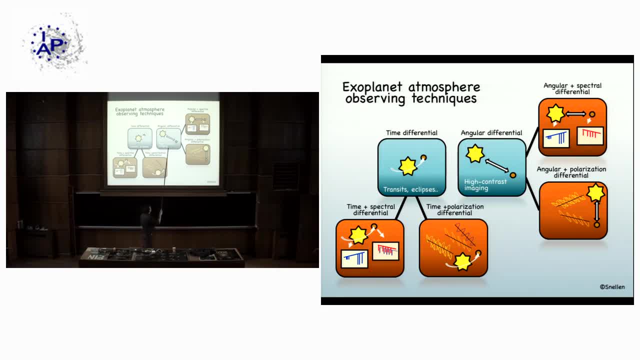 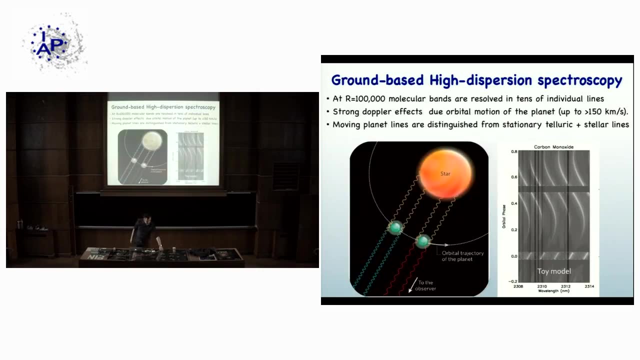 In the same way from the high contrast imaging, because these two spectra are different. you can actually use that to probe much deeper into the stellar halo, And I'll show you later some actual examples of this. So how does this exactly work? So, with high dispersion spectroscopy? 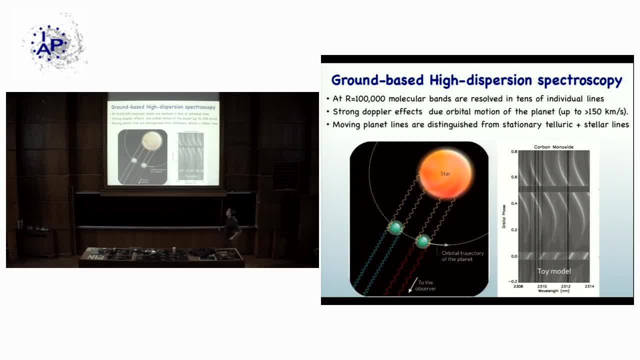 I mean, we typically work with resolving powers of about 100,000. And when we probe then a molecular band, we don't probe the band as such, but it's really we resolve the band into tens or even hundreds of individual bands or individual lines. 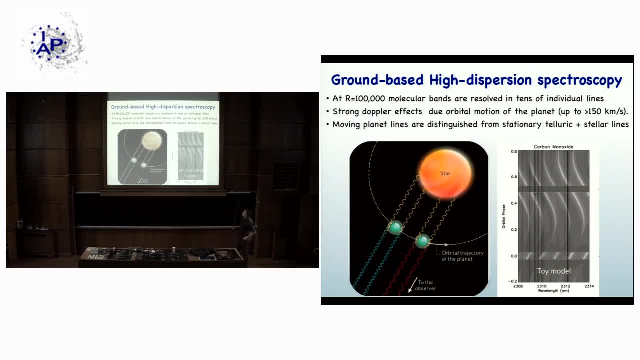 And what is important, we then become sensitive to strong Doppler effects due to the orbital motion of the planet. So we're not talking about the Doppler wobble of the actual star, which can be tens of meters per second. No, we're talking. 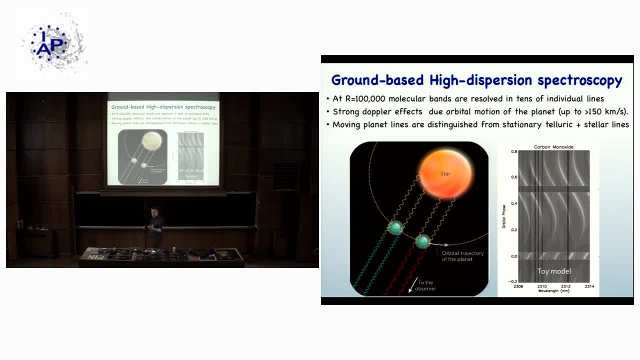 about the radial, the orbital velocity of the planet. For the Earth, this is 30 kilometers per second. For Hot Jupiter, this is up to 150 kilometers per second, or even more, And what that means is if you observe a star for a couple of hours. 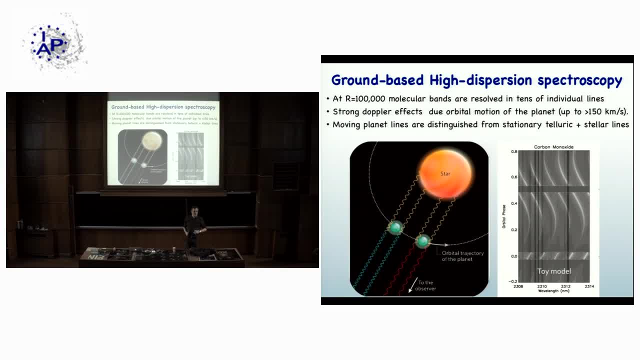 that the component of the radial velocity changes, So the Doppler effect changes and these planet lines, they move through your spectrum over the course of a night And you can use that movement to basically filter out anything else that does actually not move during the night. 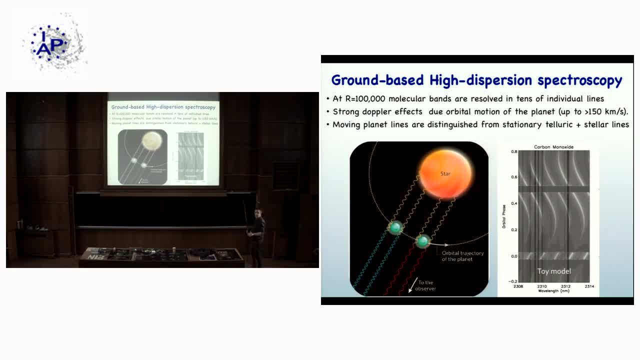 For example, the lines in our own atmospheres and any stellar lines. So this is just a toy model of carbon monoxide. how this would work. This is orbital phase and this is wavelength. And this is the light and white are the planet lines. 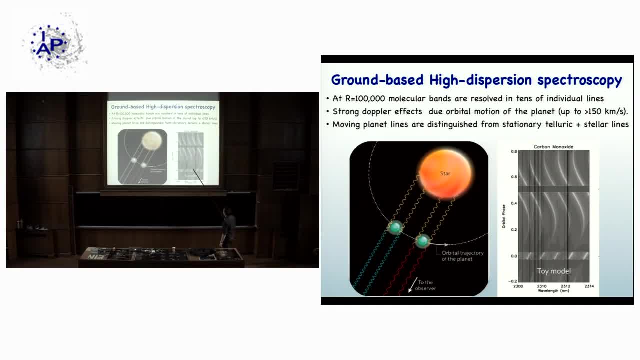 So they change in radial velocity. Here is the transit data. Here is the thermal emission data. You don't see it here because normally the night side is cooler. Therefore the lines are much weaker, And what you also see during the secondary eclipse. 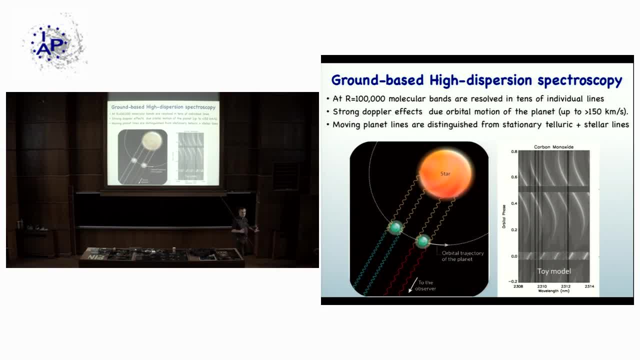 yeah, you don't see any planet light. So, although before, like the, James Webb and Ariel will really use the fact that you have planet light just before and after the secondary eclipse, and not during the eclipse, to measure the planet light In this case, 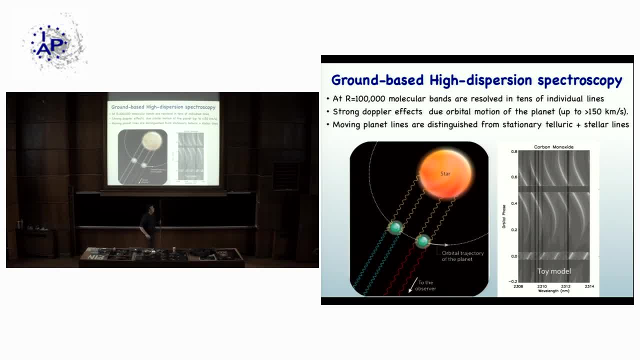 you actually cannot use the secondary eclipse light And therefore we don't have to do this for only transiting planets. We can basically do this method for any planet that is bright enough. The first example I want to give is of a transit spectrum. 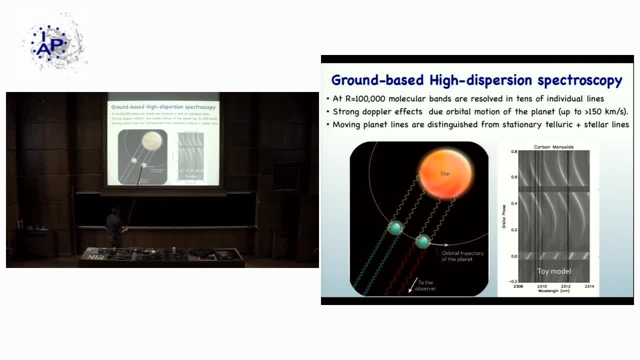 So why is this slanted? Well, when now, if we take the orientation in such a way, you have the star here, the planet, the Earth is in this direction. When the planet moves in front of the star, it doesn't do that. 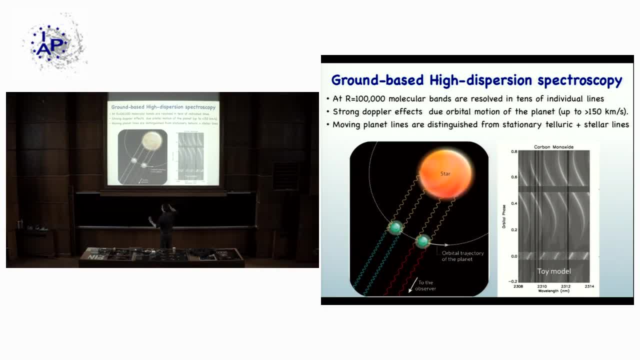 in an actual straight line. The orbit is a bit curved, meaning that in the beginning of the transit the light is a little bit blue, shifted, because the star is moving towards you or the planet is moving towards you And the planet is moving a little bit away from you. 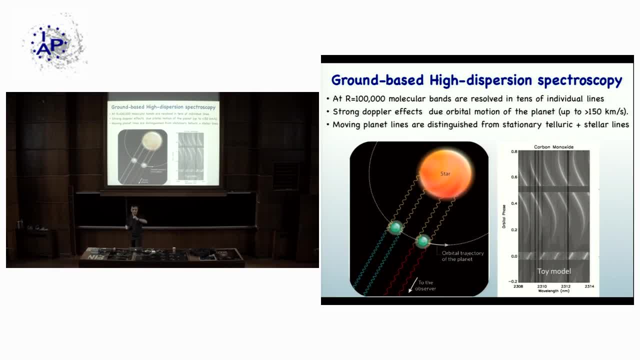 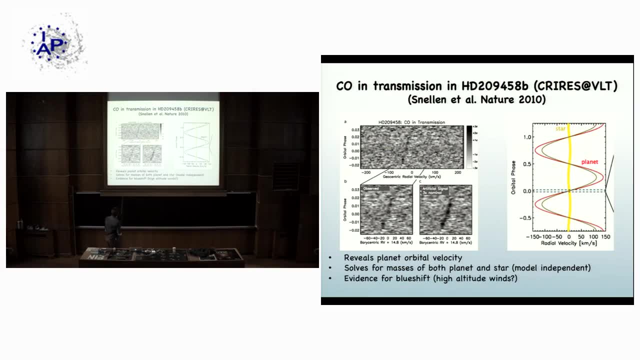 And that's why this line is slanted, And the way it's orientated tells us what the orbital velocity of this planet is. So we did this already a couple of years ago And this is now. So what we do is we try to actually remove. 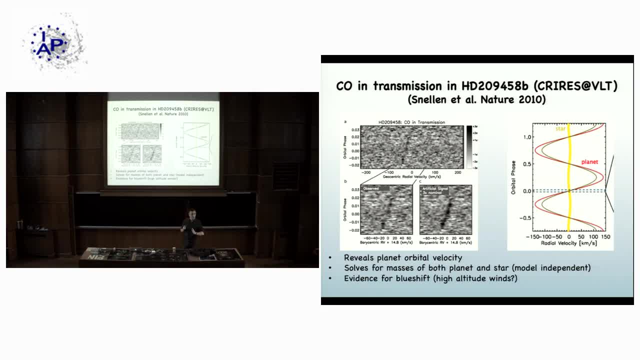 any stationary part of the exospectrum. We have a residual spectrum as a function of time And in that we have a cross-correlation method to search for the CO lines in the exospectrum and add up the signal from all the individual lines. 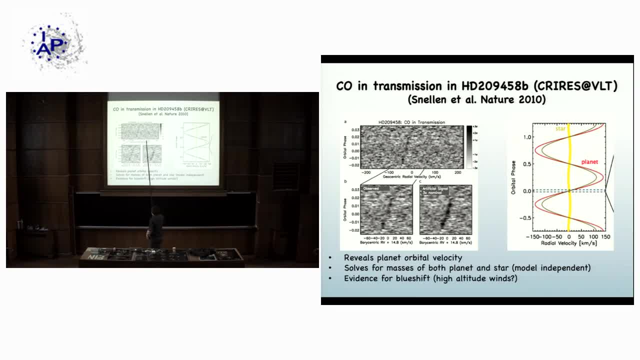 And this is what you basically see. This is the cross-correlation signal as a function of velocity and as a function of time, of orbital phase. And you see already there's a faint hint here: This is offset from zero, And that's because 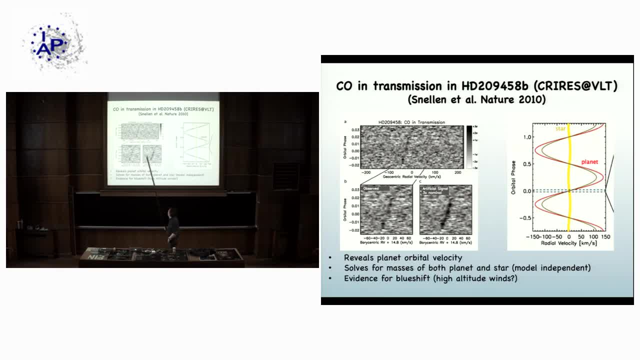 of the system velocity of the star and the barycentric velocity of the Earth. If you then put it in the rest frame of the star, you get actually this, And you get indeed this actually slanted line. And what is now nice? 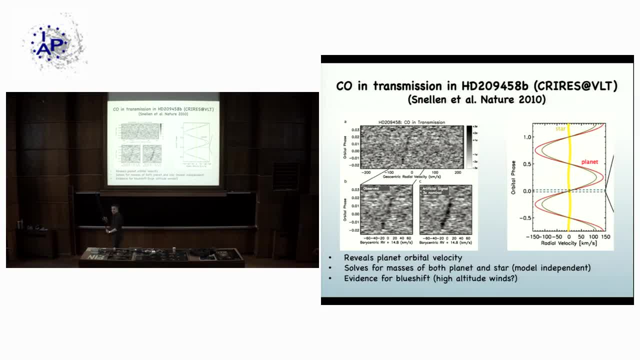 is that this orientation gives you the actual velocity of the planet around the star, And because we already had before measurements a decade earlier, of the orbit of the star around the barycenter itself, so we now have the velocity of both the star and the planet. 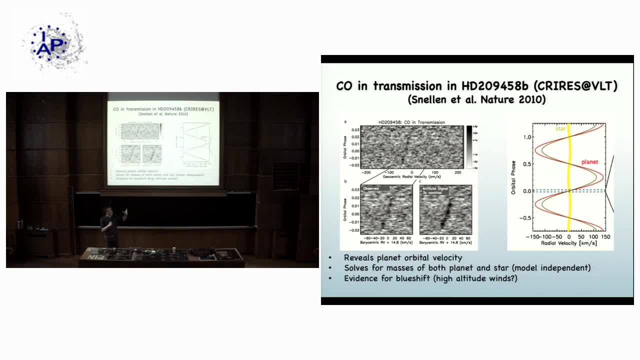 meaning this is basically now a spectroscopic binary. You have the velocities of both stars and therefore you can solve for the masses of both planet and star only using Newton's laws. Also, what we see is that this is a small average. This is only a two-sigma measurement. 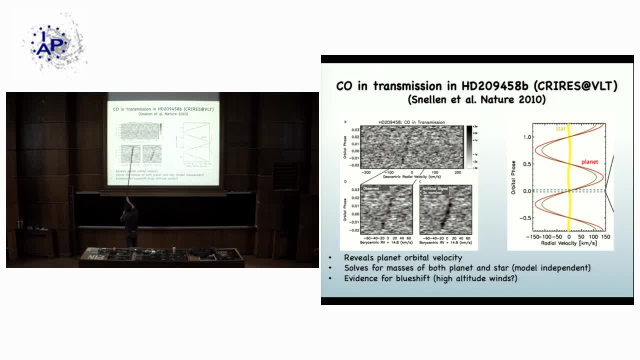 There has been more recent work of other groups, We see that actually this signal is a little bit blue-shifted, by about two kilometers per second with respect to the rest frame of the star, And we think, although the evidence is weak in this case, 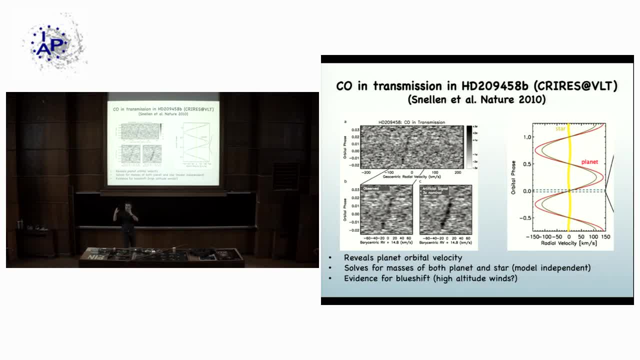 that this is caused by when this planet moves in front of the star. if this is the star, then the hot day side is on this side, the cold night side is on that side and we probe an annulus of atmosphere. And because it's warm here. 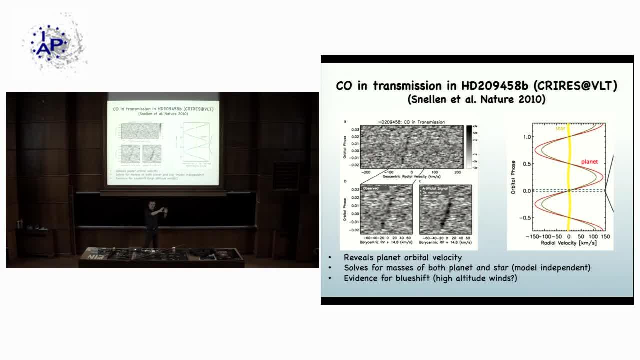 and cold. there you actually expect a global wind blowing from the hot day side to the cooler night side, giving a blue shift in the ring of the atmosphere that we actually observe. But this is also the first evidence of seeing some of the atmospheric dynamics. 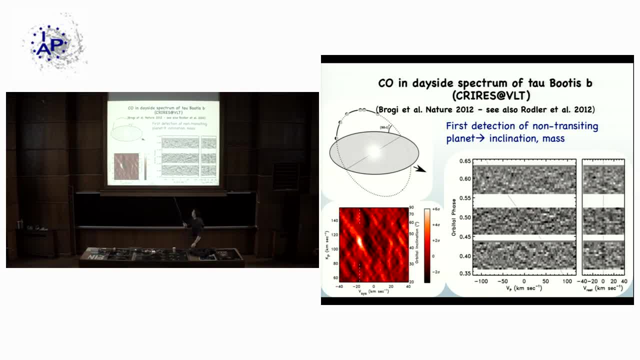 of this system. What we did here is then. so this was for the transit measurement. Now we went for thermal emission. As I already explained, we don't need a transiting system, and that's good because we can go to a more nearby system. 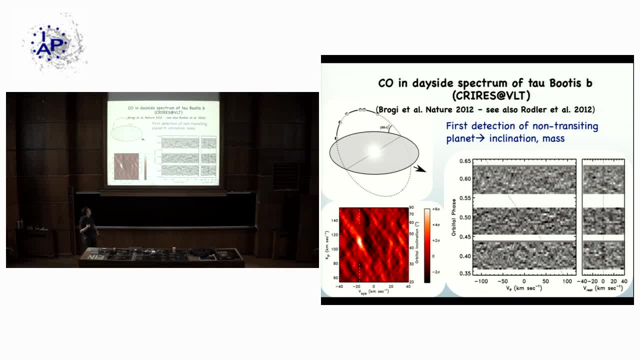 This is the most nearby hot Jupiter. we can see from the VLT And basically we do the same method, but now we don't know the inclination of the system. We observed it for three nights. I think we used the VLT in the 8-meter class telescope. 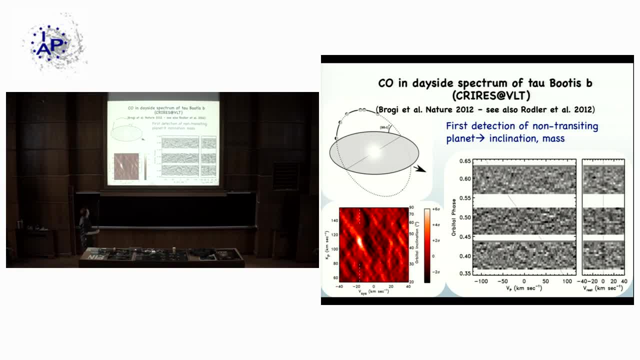 for three nights to look at the 3.5-magnitude star, And this is basically the similar diagram. This is again the cost correlation measurement as function of time. These are the three nights. This is velocity And you have to squeeze your eyes a bit. 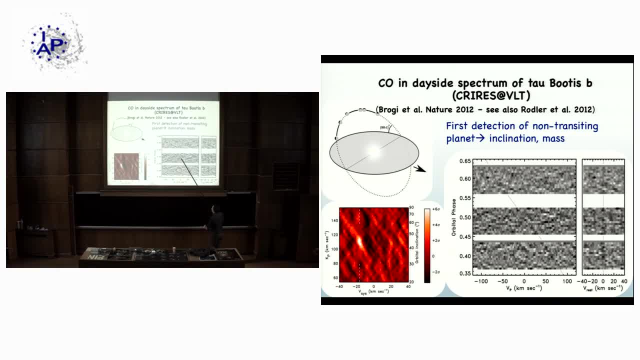 Therefore I have this guiding line, But here you can see the actual planet signal of carbon monoxide moving from about plus 80 kilometers per second to minus 80 kilometers per second around the star. You can see it better in the actual rest frame. 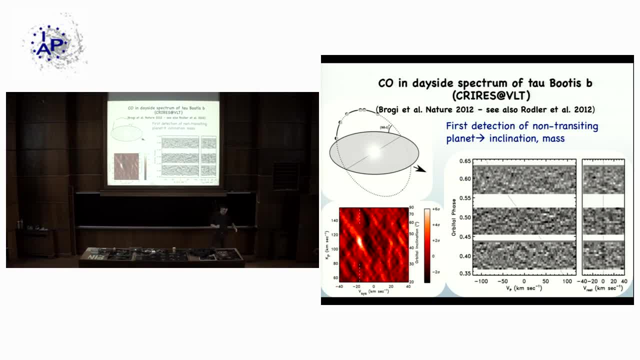 of the planet. here Now the individual spectrum gives about a measurement of about one sigma. So you want to add up the signal as function of time to really get the overall carbon monoxide signal. And the way we do that? because we don't know. 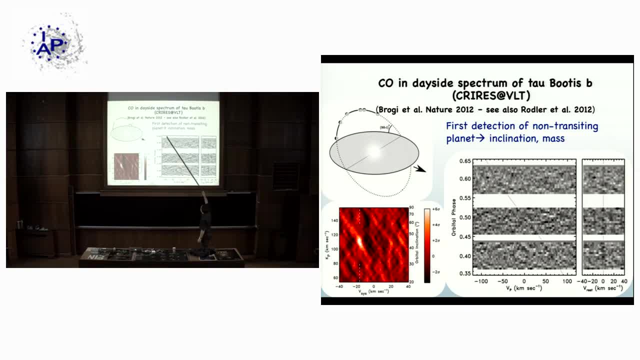 the inclination. if the inclination is very high, the change in the radial component is large. So you would expect a signal which goes like this: If it's almost a phase cycle, if it's on orbit, we get a signal which is like that: 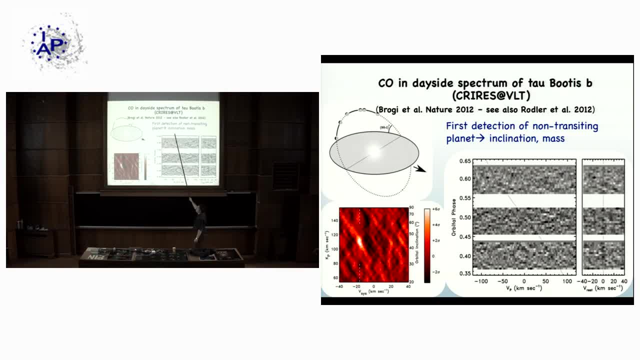 So we can add up the velocities in different ways in that way And we can presume, as if we don't know, what the system velocity of the star is. So we can add them also up in this way. So this is now for different inclinations. 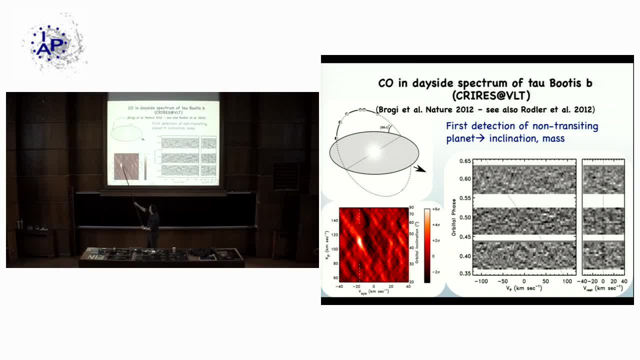 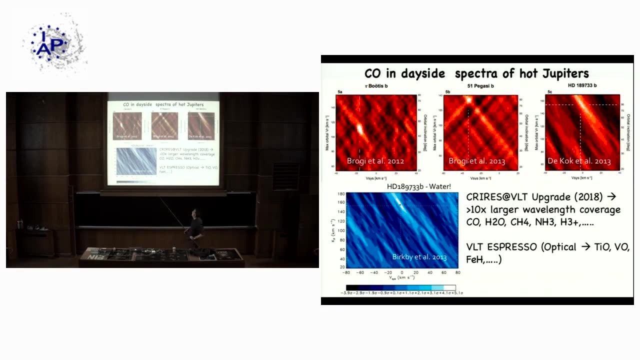 and for different system velocities. Now we see a very nice signal here. It's about six sigma And it is actually right at the known system velocity of this star. Since then we have done a handful of these hot Jupiters. 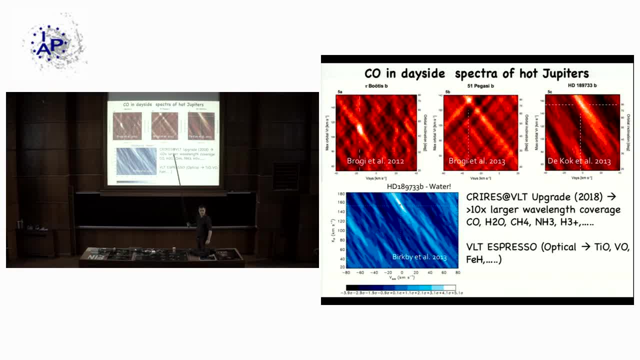 The nicest one is, of course, the mother of all exoplanets. Planets 51 Pack, It actually turns out. it has an inclination which is very high, So it's actually almost an actual transiting system. It probably only misses. 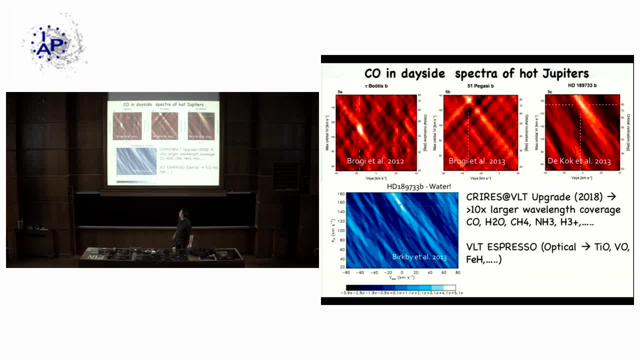 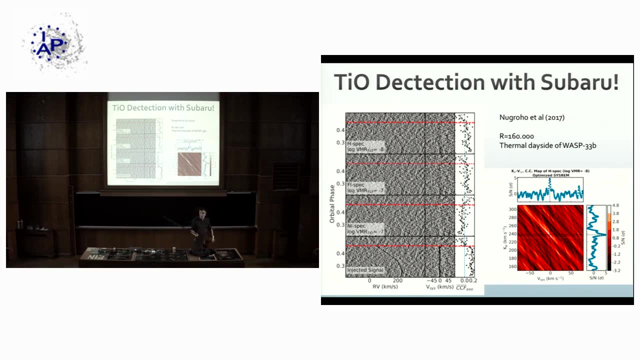 the transit by a few stellar radii. Now I don't want to go because I don't have time. I'm skipping a few things. This is a Japanese group. We have done some very nice work on TIO in the optical. 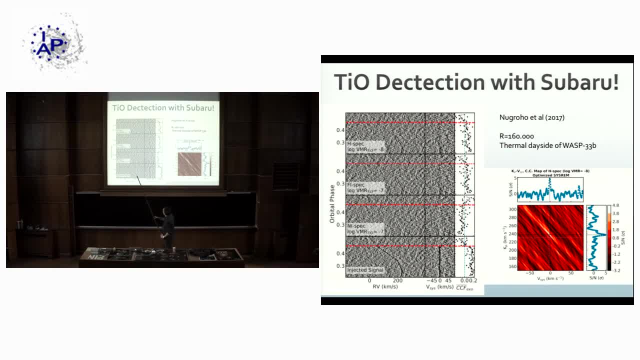 This is when you actually inject a spurious signal, a fake signal, But you can see here the actual, real signal in the data, And the nice thing is that this is actually. This molecule was expected to be present in these very hot Jupiter atmospheres. 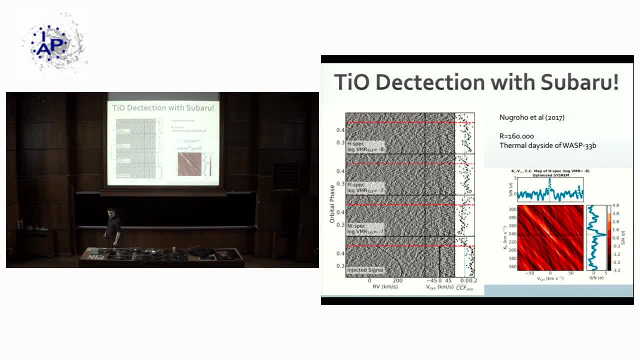 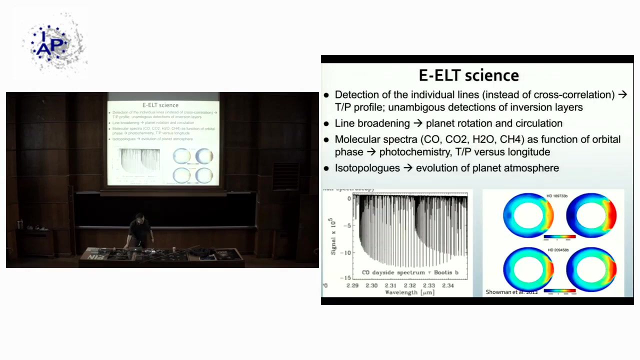 but it had never been seen. But what is very nice, you see this molecule in actual emission. So they see emission lines And that means that there is actually a thermal inversion in this very hot planet WASP-3033.. OK for the last part. 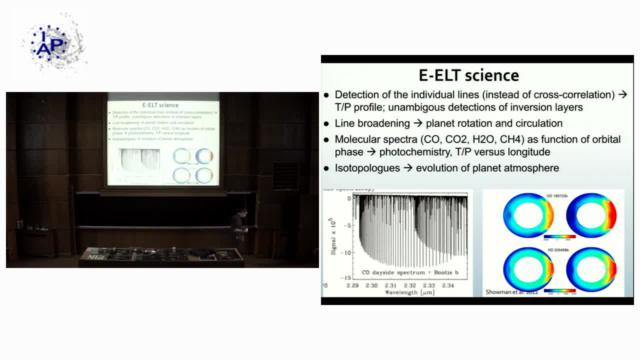 of my talk. I want to look a bit more in the future And that is really as I just said, we use the VLT three nights to look at the 3.5 magnitude star. It shows you that this kind of science 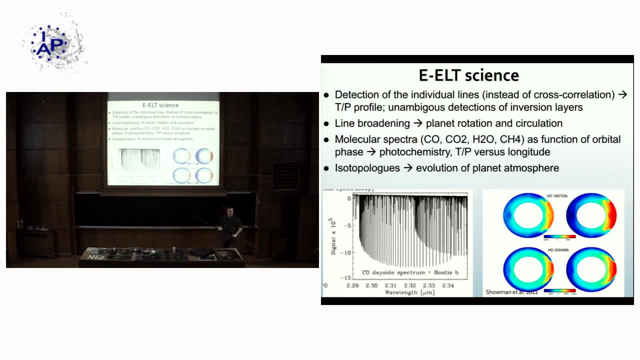 is really photon limited And a larger telescope therefore really helps. So we are very much looking forward to the ELT And there's a whole interesting suite of science cases that you can actually do. Something we have been looking into very recently is: 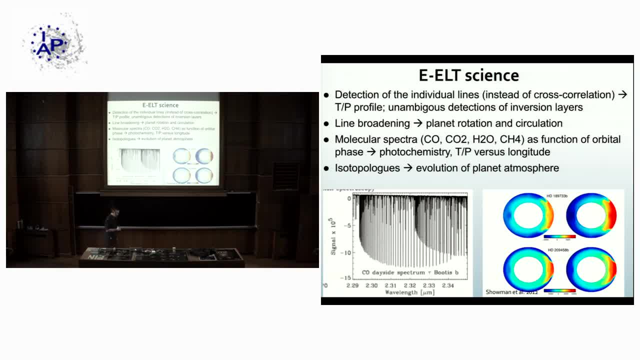 for example, what kind of isotopes can we actually look for? We are now inclined to actually say that even for Proxima b we could maybe do. for example, the HDO over water ratio. That could tell us something about the history. 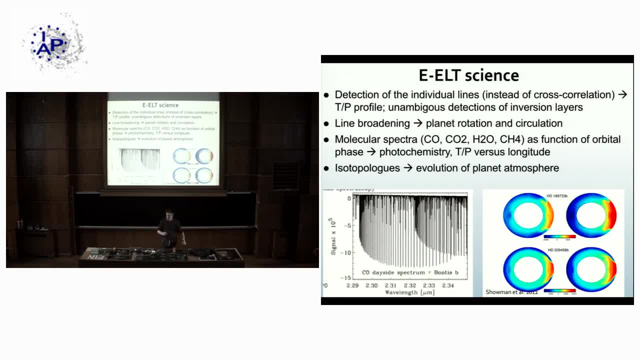 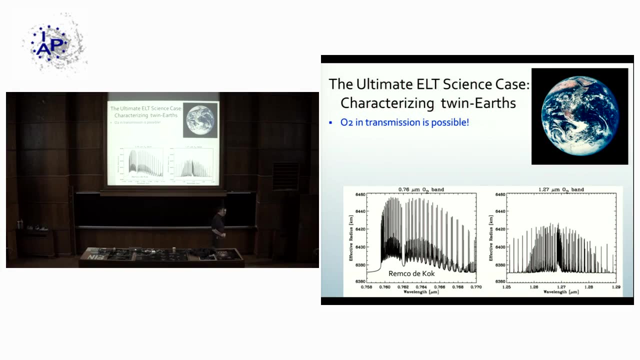 of the atmosphere and the planet. Of course, if actually water exists, we can't do anything on such a planet. But there's one science case that I want to highlight, And that is maybe the ultimate science case, and that is looking for molecular oxygen. 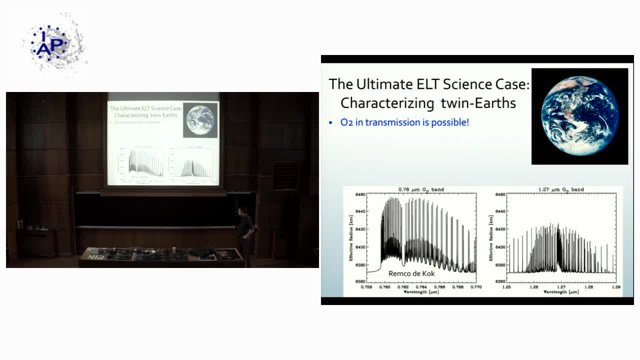 in the atmosphere of an Earth-like planet. Now, what kind of signature do you expect? Actually, oxygen is a very nice molecule to actually do this for, because it has these. it has a very nice, nice and regular spectrum. This is the 7600 angstrom band. 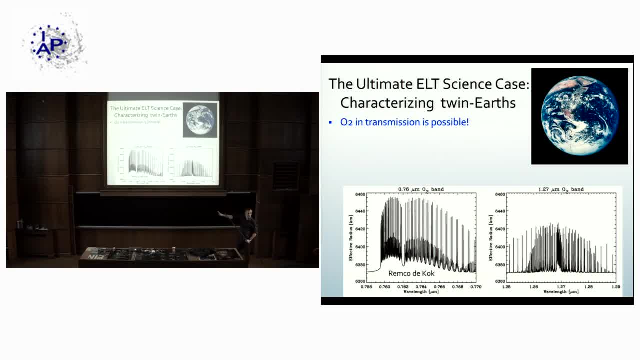 Anybody working on galaxies always thinks this is a real nuisance. It's not. It's a beautiful, beautiful band You can really use to do some very exciting science with. So you can easily calculate what if the Earth would actually transit another star. 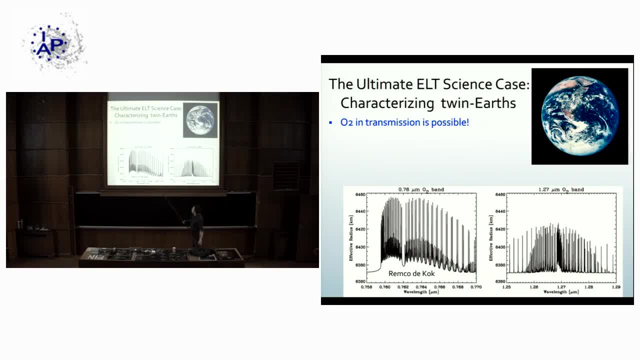 How would the? what would the absorption of oxygen look like? So this is now again the effective radius of the planet as function of wavelength, And you get typically lines or absorption would go up to about 85 kilometers And that's. I think that's the beginning. 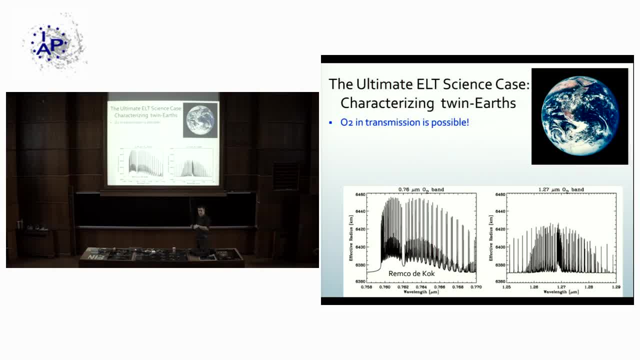 of the mesosphere where the molecular oxygen breaks up And therefore there the above, that there is no more, no more oxygen. There's also another interest. So this is 7600 angstrom. There's also the 1.3 micron. 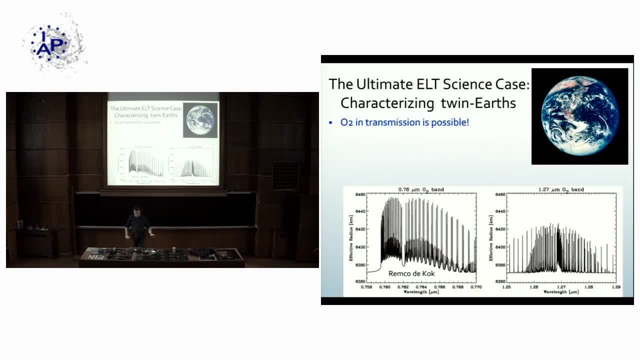 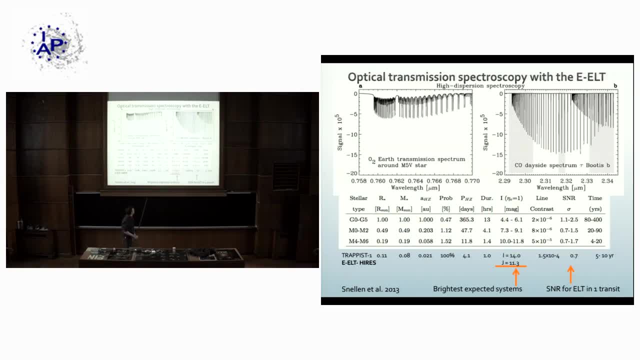 There is another oxygen band which can be very useful for the, for the redder, redder stars. So what we did a couple of years ago is to go through the numbers and see, purely from a from a photon counting point of view, what you could do with the ELT. 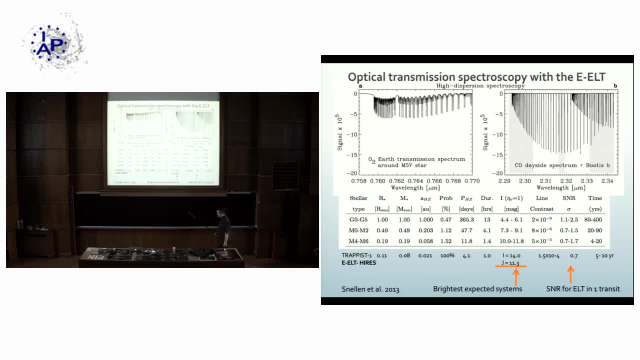 And what we did say. there is a nearby M5 dwarf, So say Proxima, like star, And it has a transiting Earth, Then what kind of? then you can calculate what this 85 kilometers in change in radius gives you in its absorption. 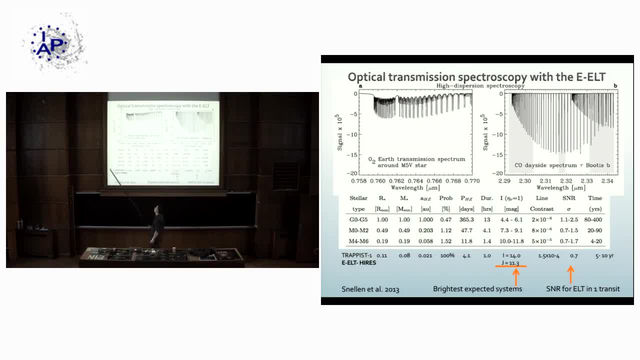 And you get signals which are about five times 10 to the minus five, And that's actually not so bad, because if you, this is a model of the CO signal we already saw in tau tau boat is B And it's about a factor 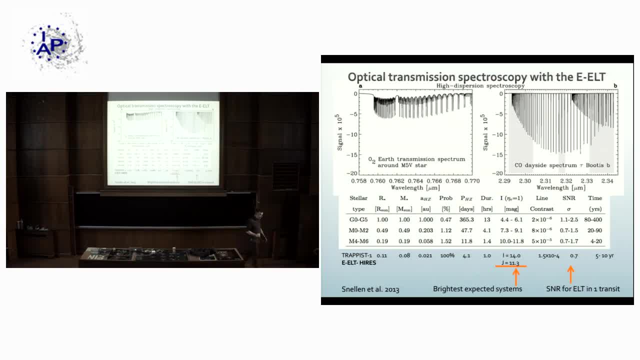 a factor three, three larger. So we only have to look for a signal which is a factor of three smaller than the signals that we actually already see. The only caveat here is this is a magnitude 3.5 star. This star will be a lot fainted. 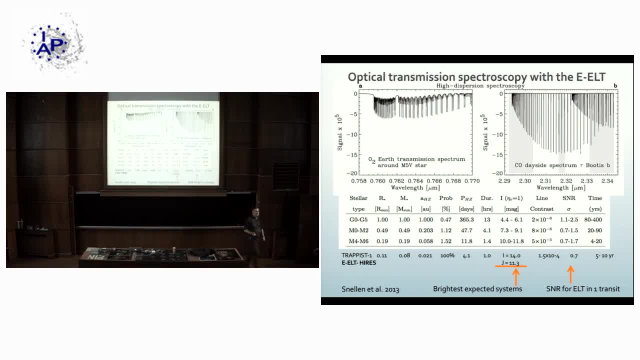 This will be magnitude 11.. So we need a much bigger telescope to actually do this And we can go through the actual numbers. So let's start here. Say that first. we assume that all stars have planets in the actual habitable zone. 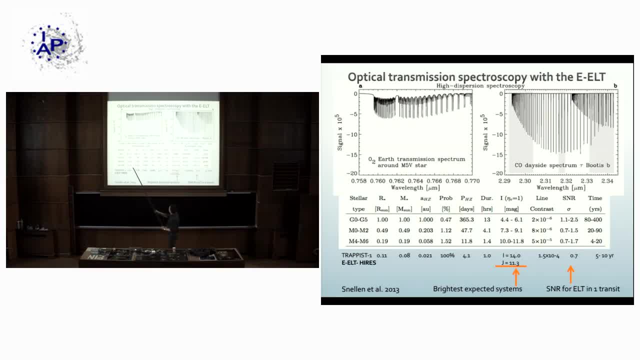 So there's kind of an upper limit. We know the radius of the star, the mass where the habitable zone is, how long a transit lasts, And also then we can calculate, we can estimate, okay, at what kind of magnitude. 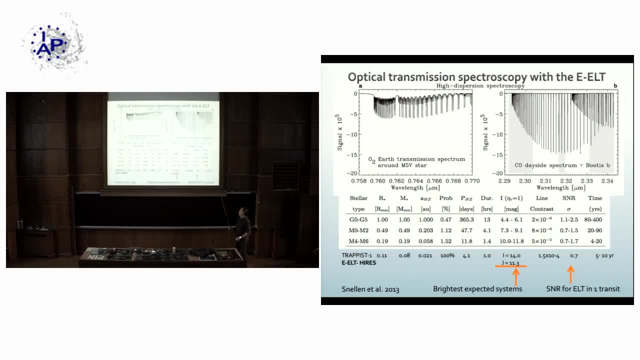 do we expect the first transiting system to actually be? No, that's four M5, that's about magnitude 11.. And what is the contrast of the lines Five times 10 to the minus five? What is the signal to noise? 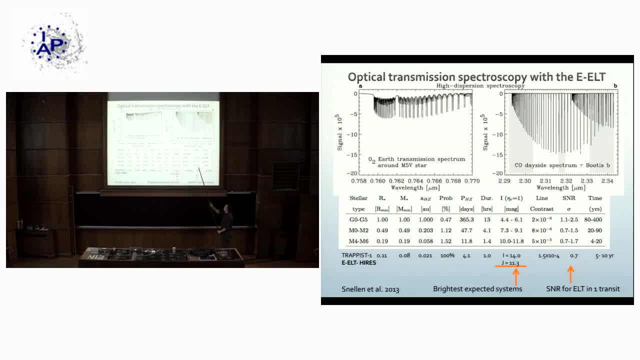 that you get with the ELT on one transit. That is actually about one, So you need to add up about 25 transits or so to see a signal, probably from one side on the earth. you can see a few transits per year. 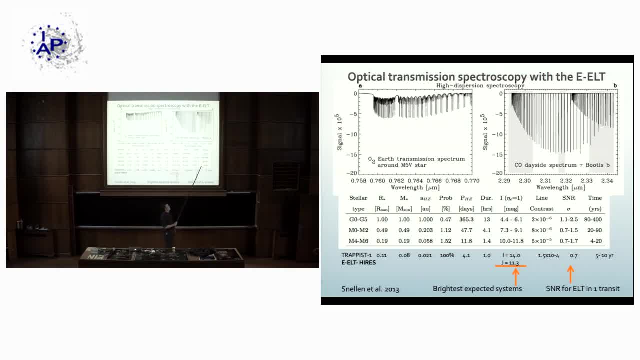 So we're talking about a project, a PhD project, of about five to say 20 years or so, So this is sort of at the limit what you could do, I think. So this is not a decade of observing time. This is during the course. 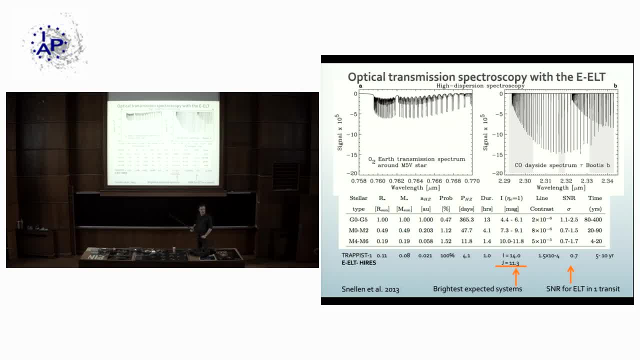 of a decade, 25 nights of actually observing time. Okay, Now what? you can also immediately see if you go to sunlight stars. actually, the stars are much brighter but the contrast of the lines are much smaller, but the signal to noise that you get per transit 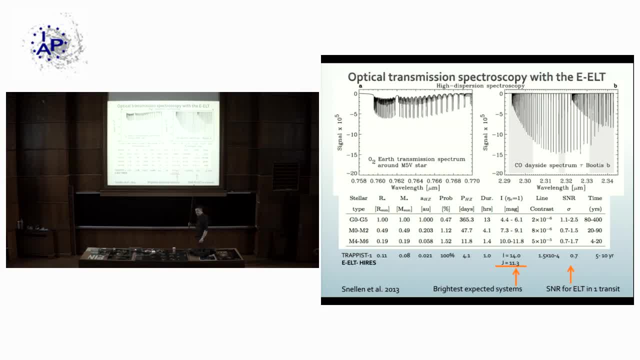 is about the same. But yeah, transits only happen once a year. You have to be lucky that the transit happens just when the sun is down, the star is up and it's not actually clouded here, So you need about 100 years. 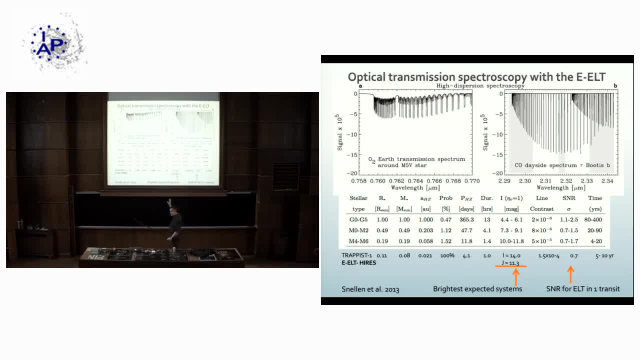 to actually get to. So this is: I think it's really out of the question that you can do this kind of transit search for molecular oxygen on solar type stars. Now, recently we have now, of course, we have now objects, For example, 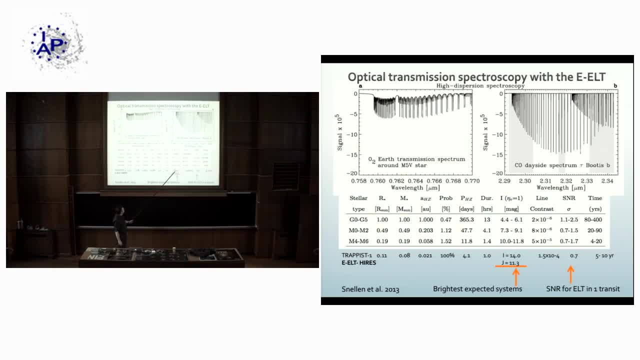 the TRAPPIST-1.. It's a bit faint a star, but the actual star is significantly smaller than an M5. So the signal is higher. The signal to noise is a little bit lower than one, So we would need about. 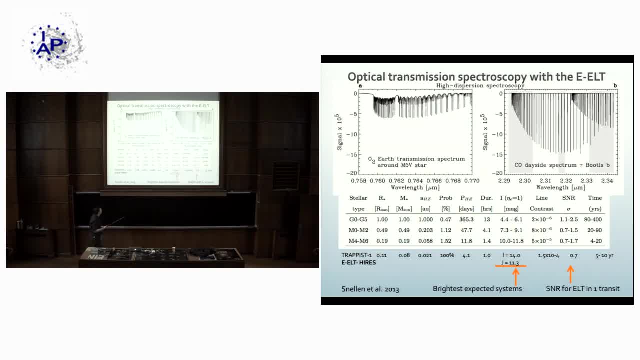 a five to 10 year project to actually do this, But I haven't gone through the numbers yet. but actually this other oxygen band is probably better because the star is actually a factor of 10 brighter, So we can actually make this a bit shorter. 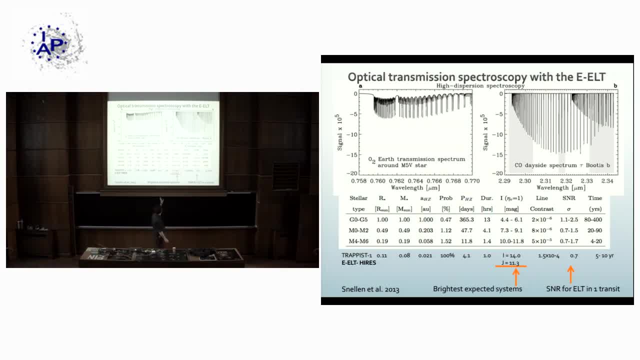 So I think actually that the ELT, when it would have a high resolution spectrograph in the optical, for example, high res- that maybe in a few years, adding up the exotransit signal, we would be able to be sensitive to actually molecular oxygen. 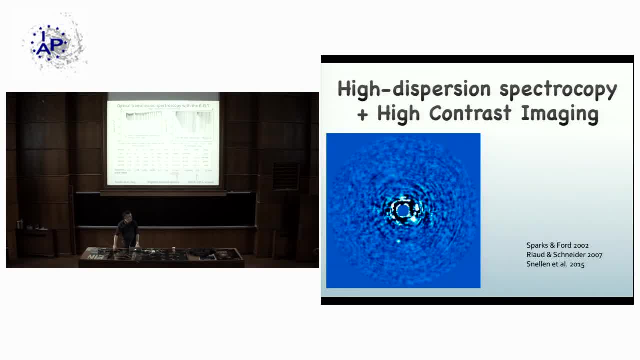 in this system. Okay, How long do I have left Matt? About five minutes or so, Five minutes. I go really fast. now for the last bit, And that is so. I talked about the high dispersion work with exotransits. 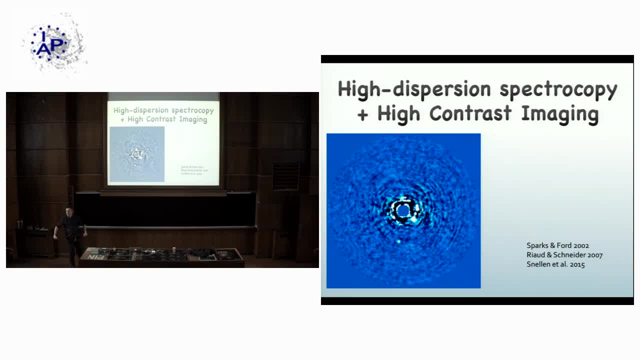 Now I want to add, to end with the high dispersion work with direct imaging. So what is the idea? The idea turns out to be quite old already. Sparks and Fords in 2002 already worked on this actual idea. What this idea is. 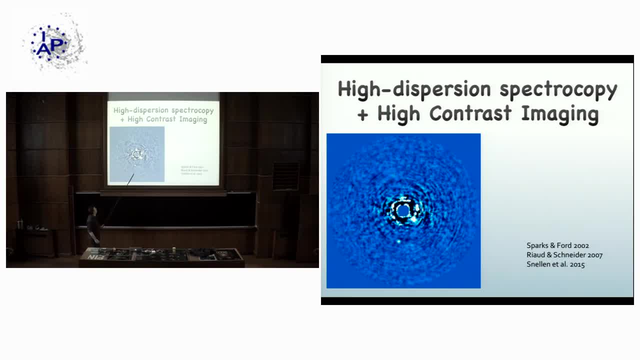 is as follows. So this is a direct image I got from Google. Here is the planet, But you see all these blobs here which come from the exostar. But yeah, you would really would like to find planets here, But it's very difficult. 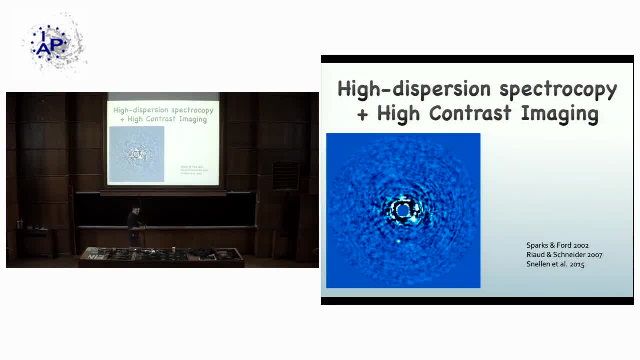 to see difference between these speckles and an actual planet. However, if you have spectral information, then actually you would see what light is coming from the star and what light is coming from the planet, Because the star in general, the starlight, will have. 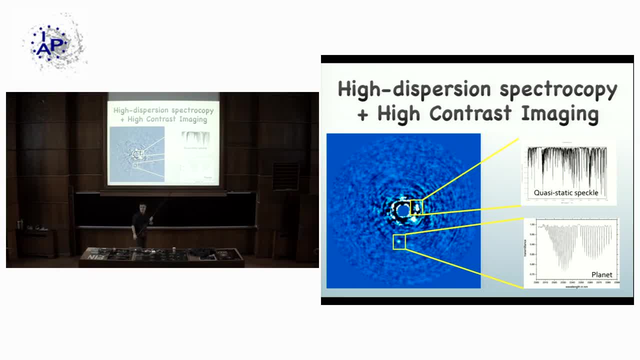 a very different spectrum from the actual planet light. So we can use that to probe down into this stellar halo and search for a planet spectrum light that basically looks like the. you know that looks like the spectrum that you actually expect. So just to show. 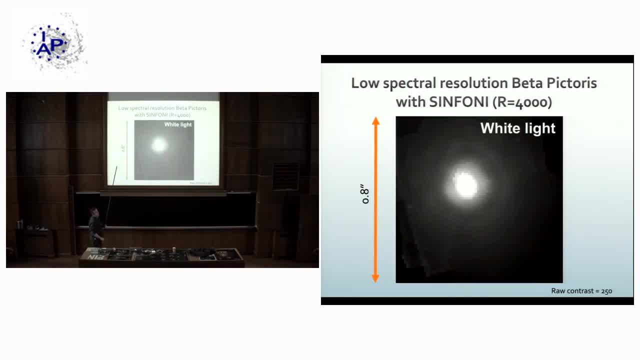 an example of this. this is one of the most famous directly image planets- Beta and PIC- And I showed an example for a resolution which is much smaller, at 4,000.. And that's because, yeah, we don't have integral field units yet. 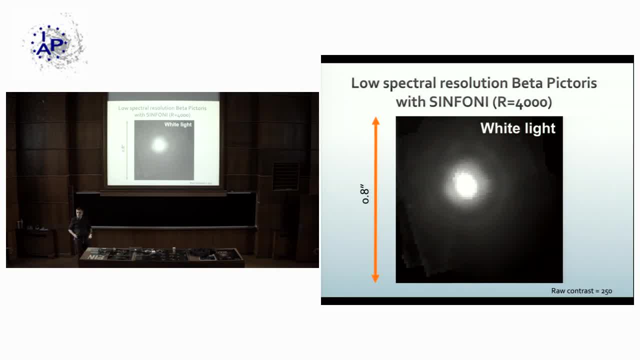 at a resolution of 100 to 1,000 that can do this. But in the future MATIS, one of the three first light instruments on the ELT, will have a resolution of 100,000.. So that instrument will be able. 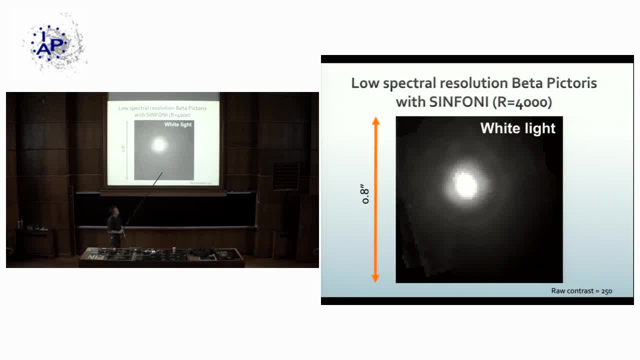 to actually do that. So this is the white light image. Actually, the adaptive optics system of Symphony is not so good. The planet is somewhere here, but it's completely swarmed by the actual star light. But we do have spectra of all these pixels. 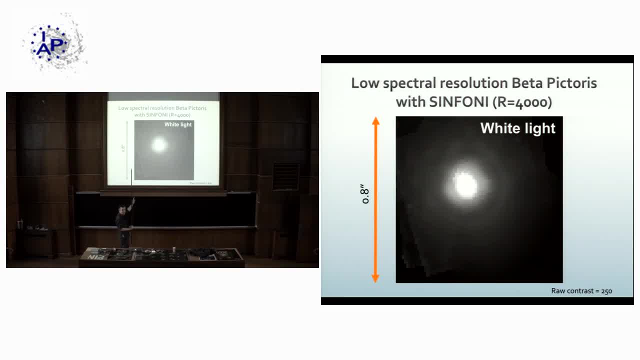 And we know the star spectrum very well, because it should be everywhere the same. So what we do? we actually remove everywhere the star light And in the residual spectrum we cross-correlate with the expected planet spectrum for Beta PIC And what you then get. 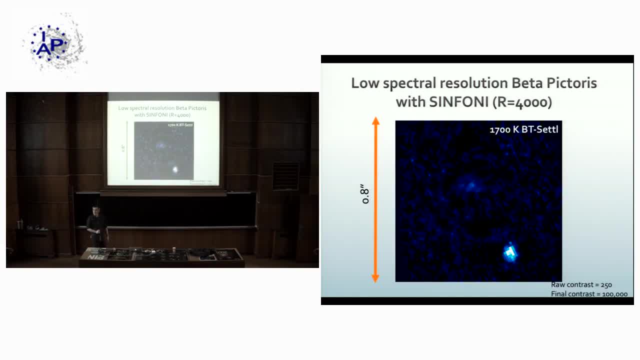 is this bit of magic? This is where planet light seems to be hiding And you see, very nice, the Beta PIC planet coming out. The contrast changes from 250 to about 100,000.. What we also see- this is for a specific model. 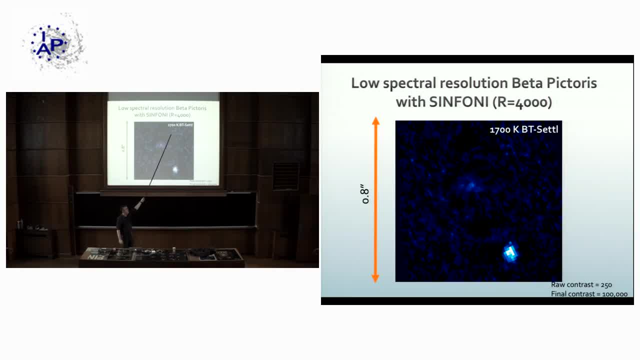 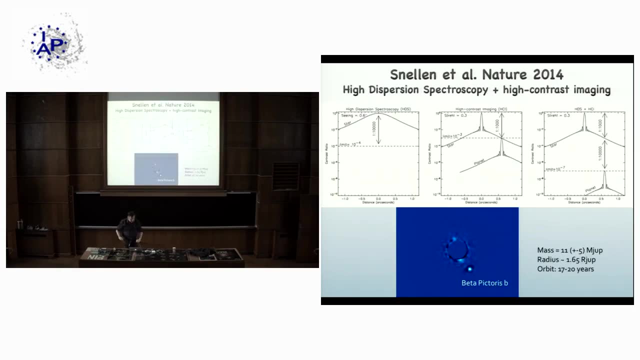 which is closest to what we expect for the exoplanet. When we move away from this model, we see the signal becoming more and more and becoming weaker, So we are also sensitive to exospecific planet parameters. Okay, so actually before that. 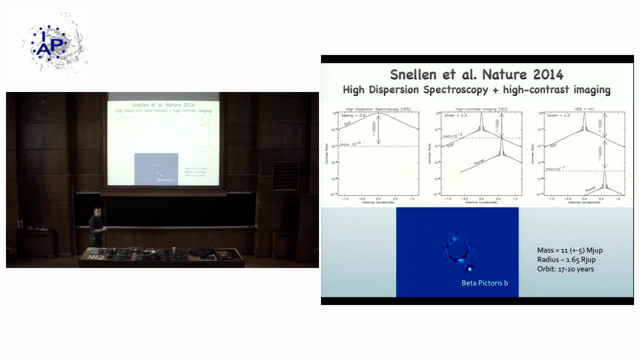 this was just an example to show how it works. Of course we don't have an integral field unit to do this at a resolution of 100,000.. But we do have the cryo-wave spectrograph with a slit. And if we know, 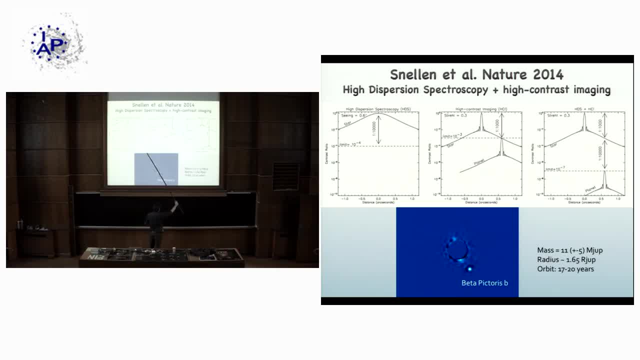 where the exoplanet is. we can just put this slit on the star and the planet and see how well it actually works. And this is a planet in an orbit about 20 years. It's about an order of magnitude more massive than Jupiter. 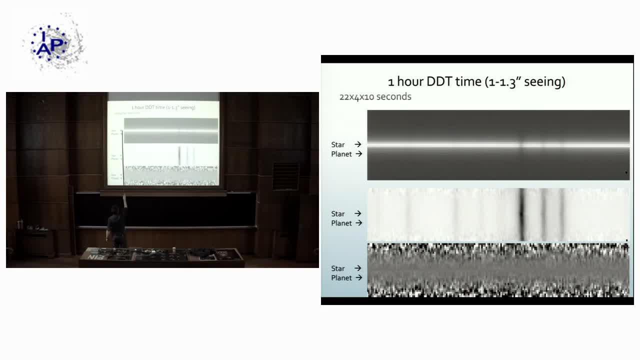 This is now the position on the exoslit. We have the star. We know where the exoplanet is. It should be here. It's completely dominated again by the starlight. We actually remove that as well as possible. These are the residual spectrum. 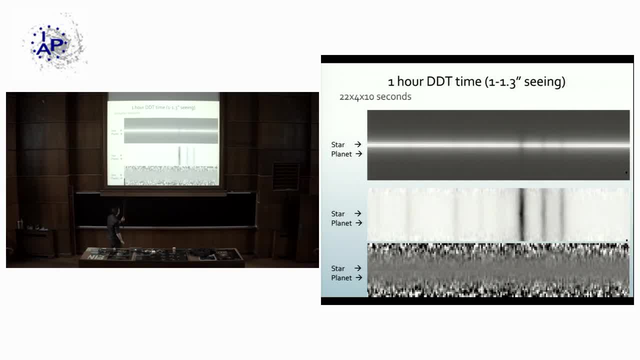 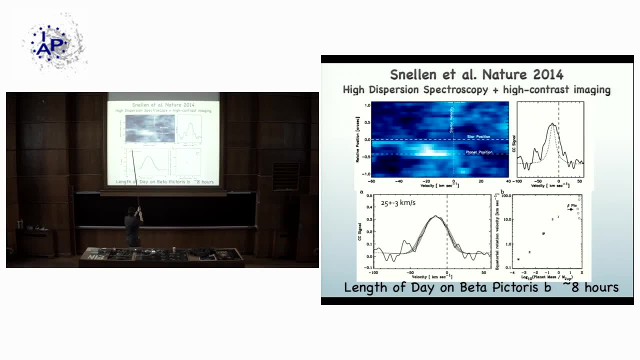 And now we cross-correlate each of these residual spectrum with a carbon monoxide template, And what we get is this: This is now the velocity of the carbon monoxide. This is the position on the slit At the star position. we don't see anything. 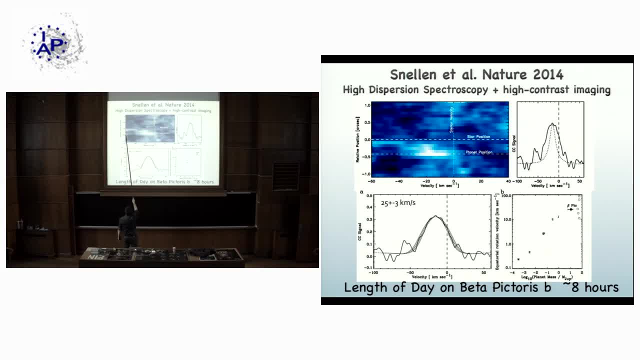 Of course, we have actually removed everything from the star. At the planet position, we see a very clear carbon monoxide signal. First of all, it is redshifted by about 15 kilometers per second. That's the orbital motion of the planet. 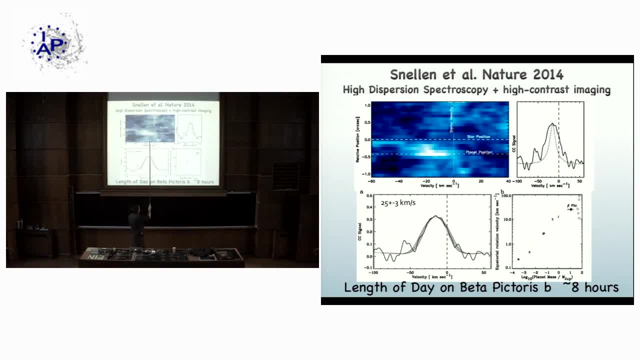 around the star And what we see is that the carbon monoxide signal is quite broad. It's broadened by about 25 kilometers per second And we think this is due to the spin velocity of the planet. That's because of the rotation. 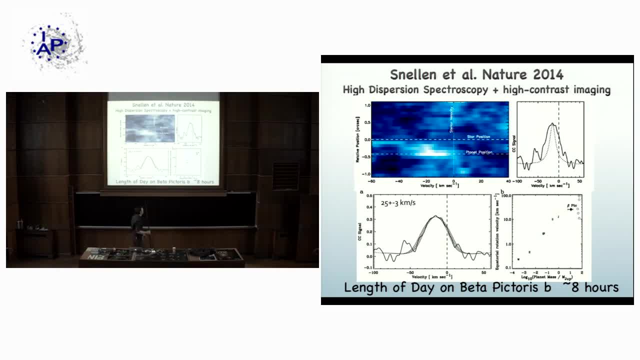 of the planet And because we sort of know what the radius is, we can derive that the length of day on Beta Pictoris is about 8 hours. This is a very fast rotation, But if you look at the planet's mass in the solar system, 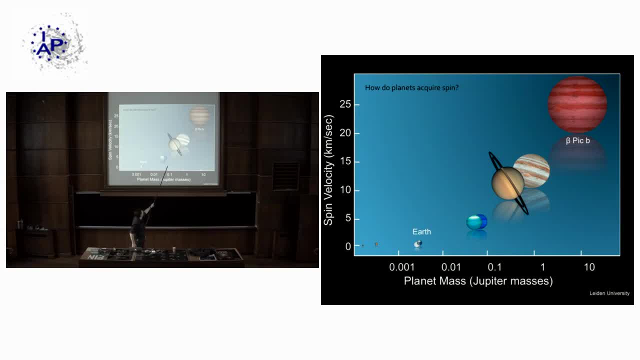 as a function of the spin velocity. you see, there is actually an actual relation And Beta Pictoris just extends this relation to actually the higher masses. This is some ideas we have about how planets can actually get spin, but I don't have time. 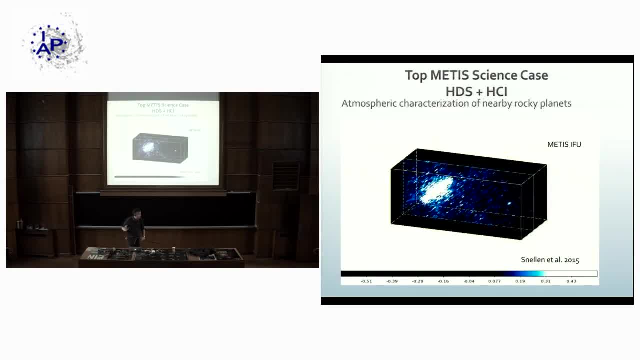 You can ask me later, But one of the top science cases for METIS is to actually do this on nearby planets, So we can really push this to rocky planets As an example. this is one night of observing of a super earth. If Alpha Sun would have. 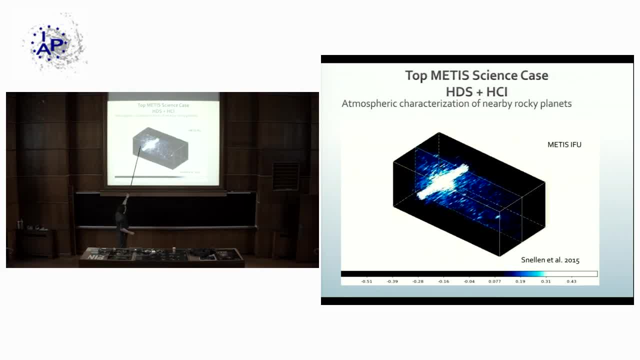 a super earth. what we now have this is the eye view of METIS. We have the two axes here, which is the angular position on the sky, And this is velocity At the star position. it's, of course, very noisy because of all the photons. 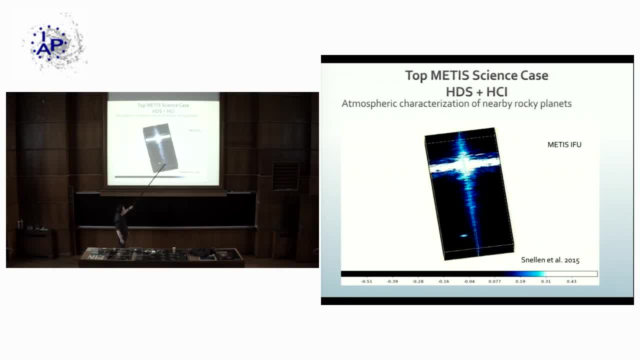 from the star, But also at velocity zero. it's very noisy And that is because we look for spectral features which are the same as the spectral features in our own atmosphere, But because of the radial velocity of the planet it's actually offsetted. 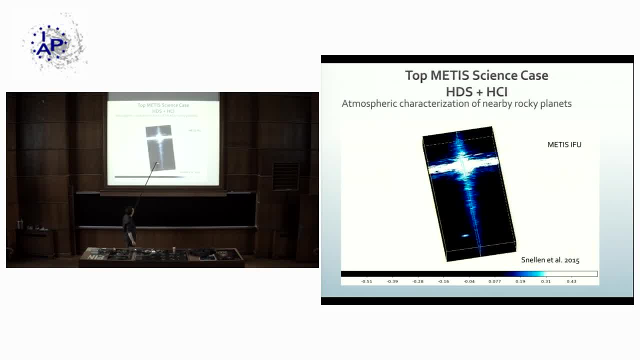 And therefore you can see the actual planet. And if we would observe now, a few months later, it would not only have moved in the sky, but also the radial velocity would have changed. So you can also map out the radial velocity orbit of this planet. 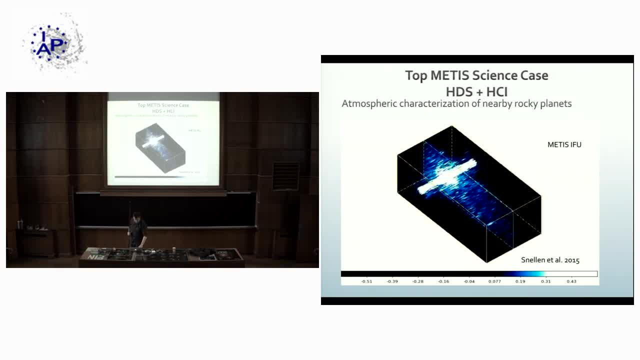 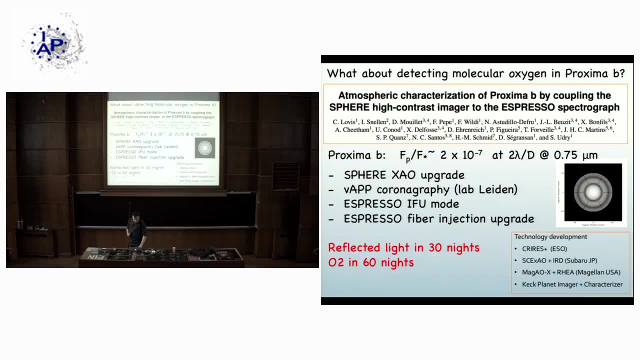 So this: with the first light instrument, METIS on the ELT, we will be able to actually do this, hopefully not long after first light. What we really want to do is to move this to the actual optical to look for reflected light. 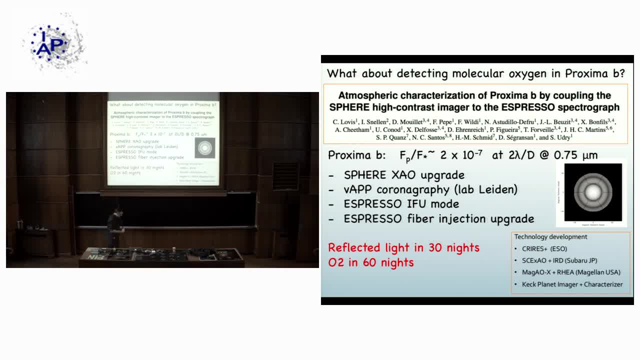 to look for oxygen, And then we really have to try to understand how to actually do this, And I think, therefore, a very important project is led by Christoph Loewis to actually try to couple the sphere instrument with actual ESPRESSO or a similar instrument. 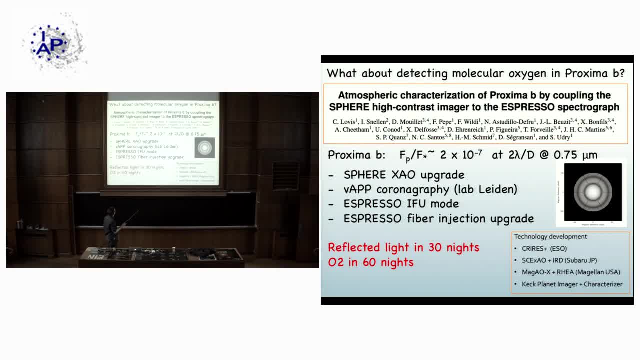 to get this high resolution capability on a sphere to actually test this, One of the things he had been going through, and I think this will be very difficult, but he claims, if we can do this well, we could actually measure reflected light on Proxima b. 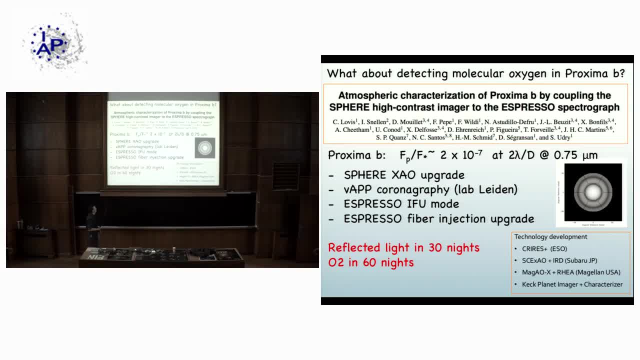 in about 30 nights. I think this will be very difficult, very challenging, but I still think it's very important because this really will teach us how to actually do this. There are a lot of different instruments, now also in Keck and Subaru. 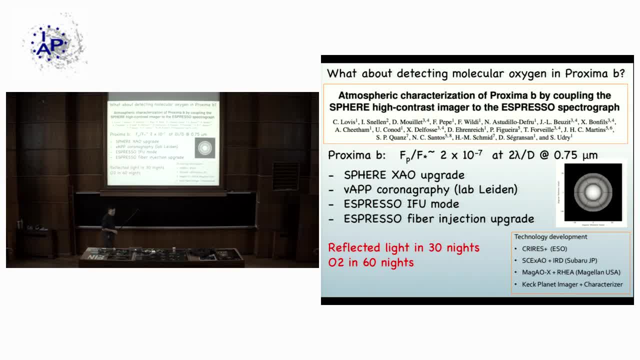 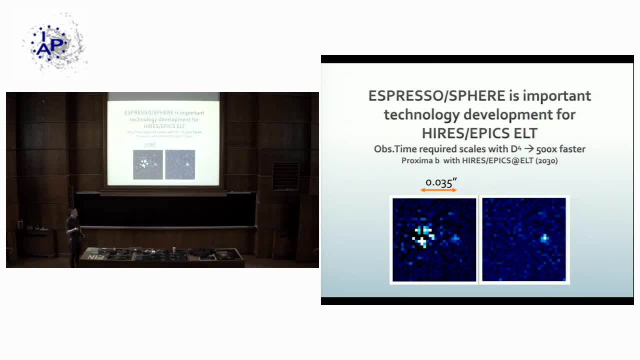 that are building instruments that are going to actually do this, And I think that's really important because you have to realize that this method scales the actual exposure time needed, scales with the diameter of the telescope to the fourth power. So if we can almost do this, 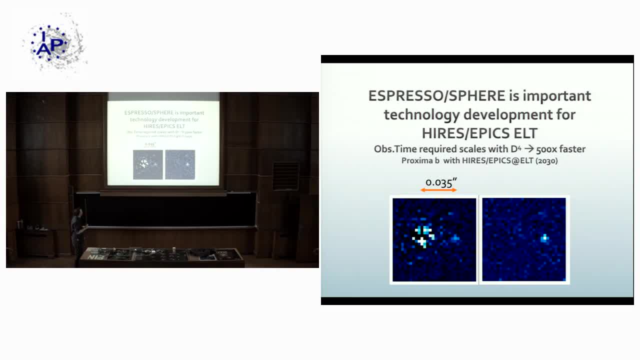 with the VLT coupling sphere to a high-dispansion spectrograph. with the ELT we could in principle do this a factor of 5,, 500 or so faster. So 50 nights suddenly only become a few hours, And then 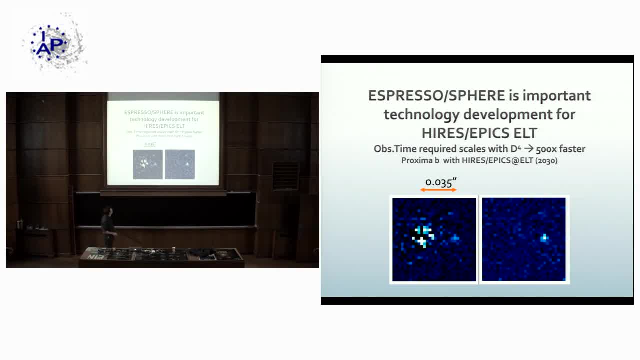 the kind of observations which you could expect. this would be Proxima b in reflected light. here is the star, here is the actual planet. So this is hopefully in the future, before I grow really gray and old, we will be able to actually do this. 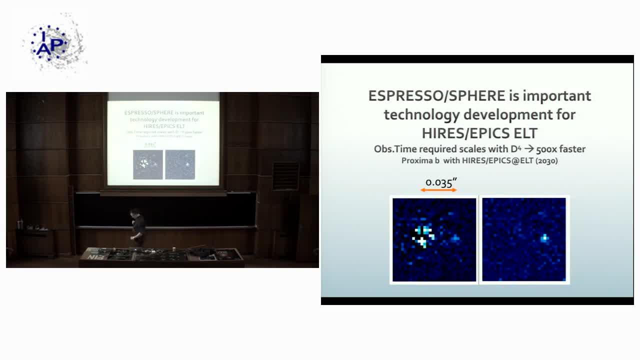 Thank you, Yeah, so super interesting. So it's interesting what you say about how it's important to collect photons. So can you just make a general comment about space-based detection of exoplanet atmospheres, perhaps with coronagraphic methods Like the terrestrial planet finder? 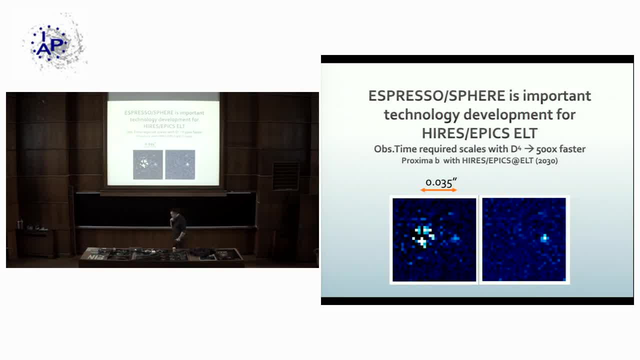 that's no longer on the cards, is it? No? no, That's no longer on the cards. So there are two new studies that NASA is doing. There is the HABEX telescope and there is the LUVOIR telescope. So one is more. 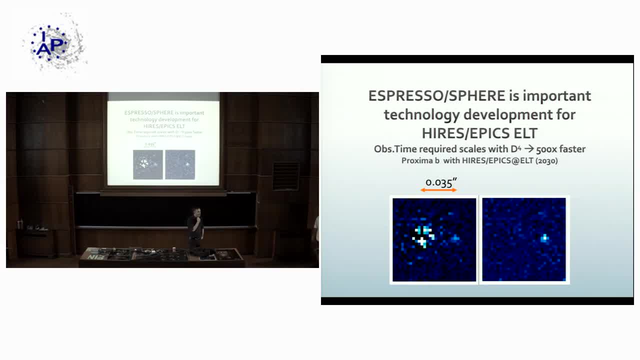 a general purpose telescope that can also do exoplanets, And HABEX is really the one that tries to only focus on exoplanets. Their wavelength ranges are slightly different. Yeah, what I think is the actual relation between the ELTs and those kind of space missions. 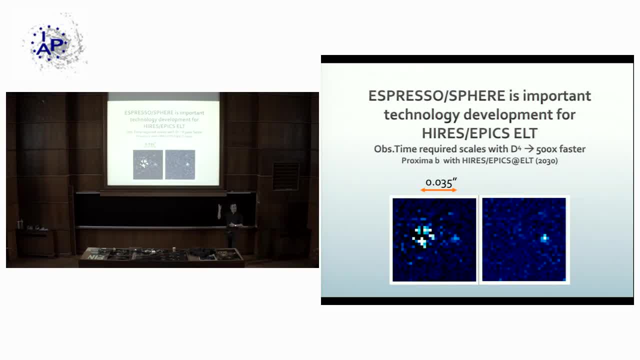 is with the ELTs, we will really do our best to try to image and to really study the most nearby planets. We will be able, for example, to do Proxima b, maybe some other very nearby M dwarfs, maybe one of the solar type stars. 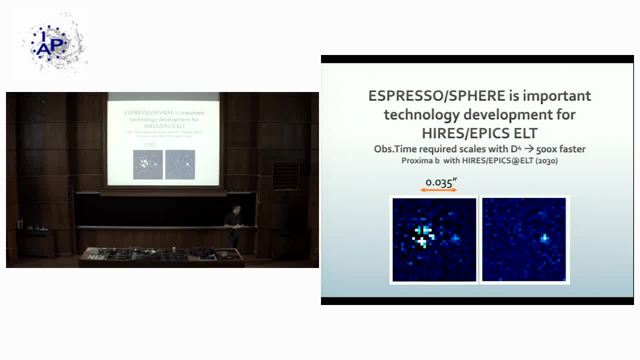 we can do one or two planets on, but it will be a very limited sample Because as soon as you go a factor two further away, factor four, fainter signal, factor 16, longer exposure- this becomes terrible. So if you then 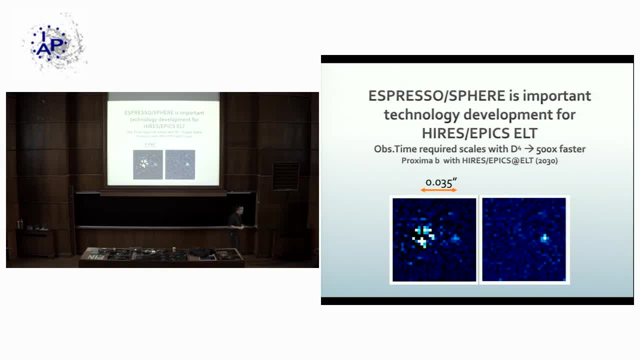 and what I started my talk with. measuring molecular oxygen is not enough. You have to understand what's happening on this planet, And for that you need to have samples of planets. So I think for the next step you really want to have a large space mission. 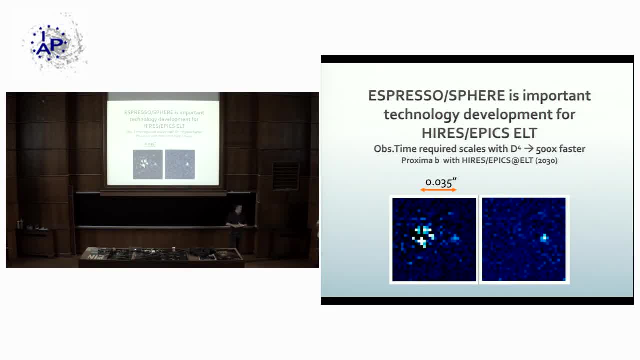 to be able to probe samples of 50 stars or so, And, for example, then the HABEX or the other one, LUVAR, could actually do this If you were observing the Earth in good condition, maybe around Proxima. 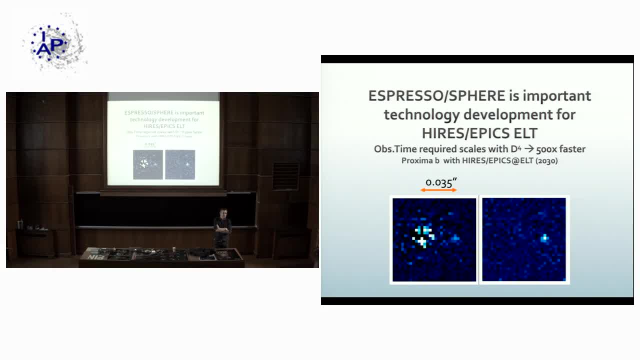 would you be able to see methane, Methane, CH4?? Yes, Yeah, I think so. that will, for example, be in the METIS wavelength range. That should be a lot of methane. So I think, for example, methane should be easier. 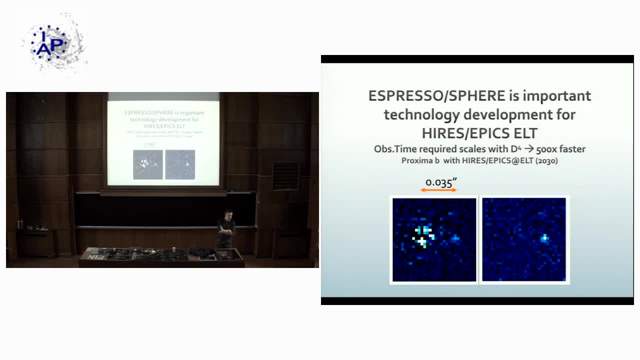 than, for example, molecular oxygen. It will be easier. Yeah, I think it will be easier if it has methane And if the absorption is strong enough. we should be able to see this, But at the level of methane in our own atmosphere. 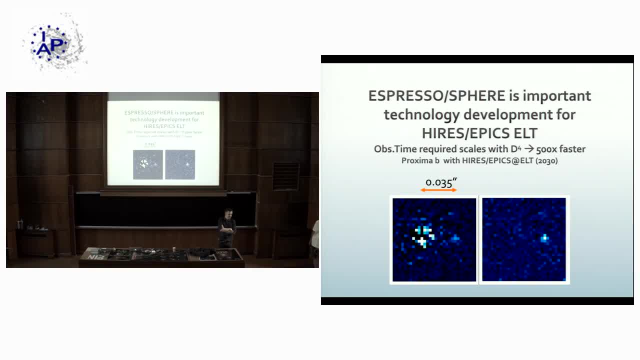 which is a few ppm only. Yeah, so, but the methane absorption is already very, very strong. So we can actually the regions where you expect the strongest methane absorption, we just cannot actually use because you don't. it's completely opaque. 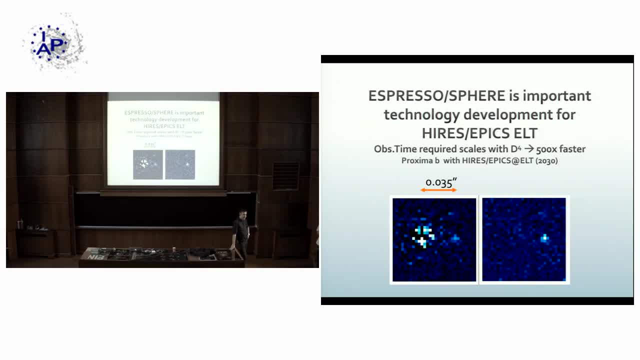 in our own atmosphere. So we actually, although the volume mixing ratio is very low, we already have to go to spectral regions where the actual absorption is weaker to be able to actually see it. But I think that molecules, like the first molecules we can do on rocky planets. 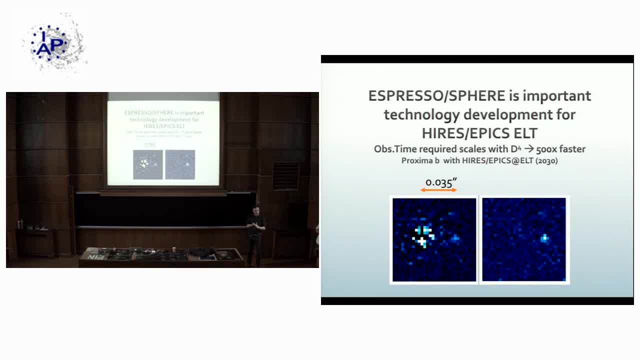 will be water, CO2 and methane. I think those will be the easier. between quotes: Yeah, And of course, molecular oxygen is more difficult because it is, it is in the optical, So any, any, yeah, adaptive optics system. 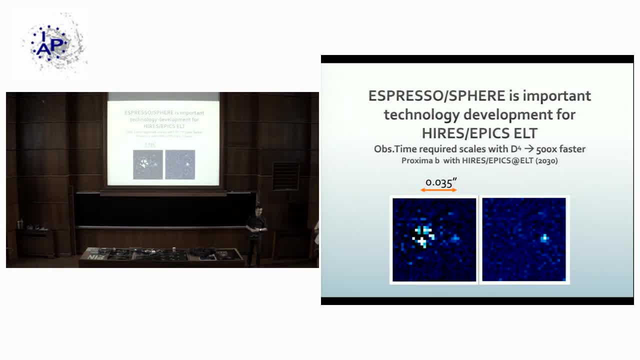 is much more difficult in the optical than we can do in the in the apparatus. Thank you, You didn't mention what you we have learned from the observation of the atmosphere of Jupiter. Have we, have you learned anything about the formation? 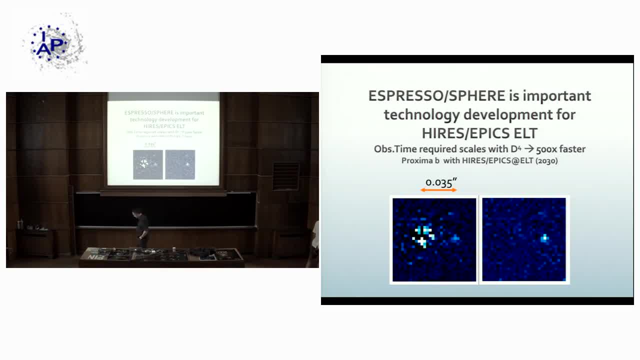 the, the history, the evolution or something, if it is possible. I know that it's probably a topic for another talk, but if you can, yeah. So you have to realize that. yeah, the first measurements on the atmospheres. 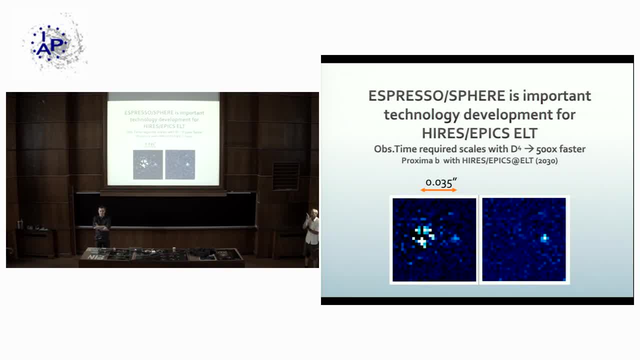 of hot, hot Jupiter's are, are, are quite recent right. So we are. we started, I think- or people started- in 2002, when they measured sodium, Yeah, And then now, since a few years. 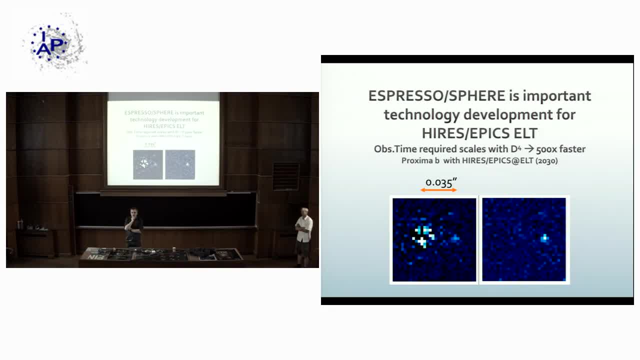 they can do water. We have some carbon monoxide measurements. All those measurements are not very surprising. There is, of course this is a hot, hydrogen dominated atmosphere. There should be water, There should be CO. So in that sense, 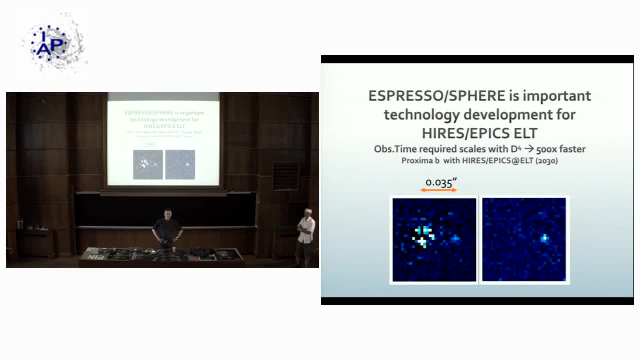 I don't think we have learned much yet really about the atmospheres or the atmospheric physics We have, I think, what I showed about David David Singh's work, about this correlation with the observation between the water signature and between the hazes. 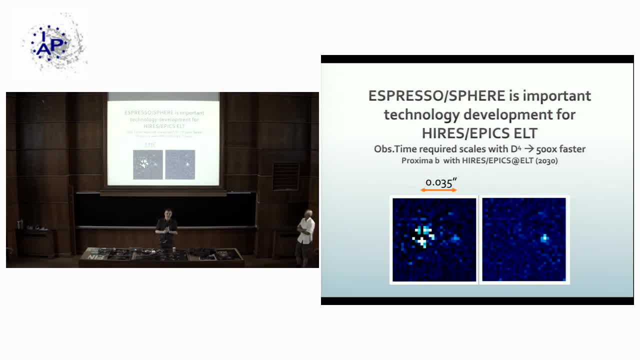 I think this is the first time that an observation is really telling us something physically what's happening in the atmosphere? Well, of course, M the dwarf stars and Brown the dwarfs have this molecule, So it's not surprising. 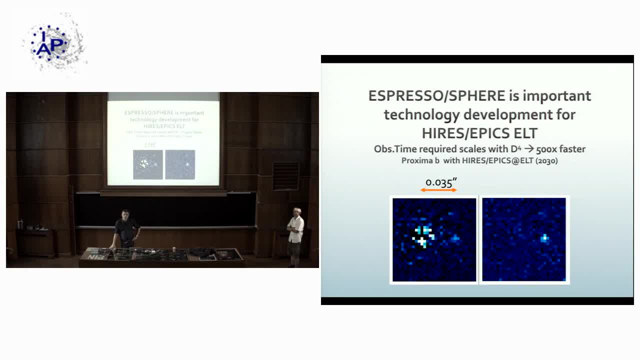 that TIO is actually present in these atmospheres. It has been searched for for a long time because there was evidence- although the evidence has been before quite weak- that these planets have inversion layers and therefore some molecule or species has to actually absorb. 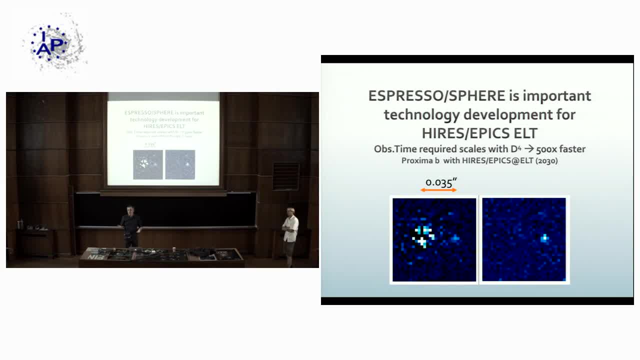 the starlight high up in the atmosphere to heat up the atmosphere. So this is the first time that we actually see this molecule. So we start to learn something about the atmospheric physics of planets, But to link that to how these planets 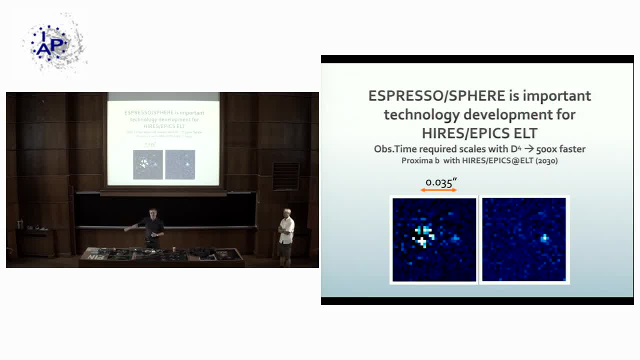 are formed. there's still a question which is much further in the future, I think. So what you have shown by using eye contrast imaging, I think, ideal situations, because we are back to what we're doing: observing the solar system. so you 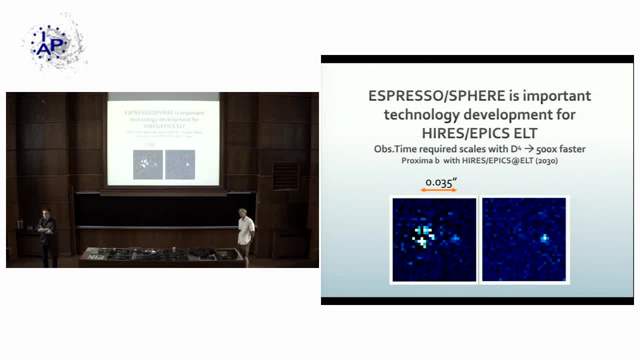 can look directly to the telescope, But we learn also many things because it's quite faint in any case. So eye spectral resolution will be always on very limited cases. So why don't use low spectral resolution or broad space, please do. 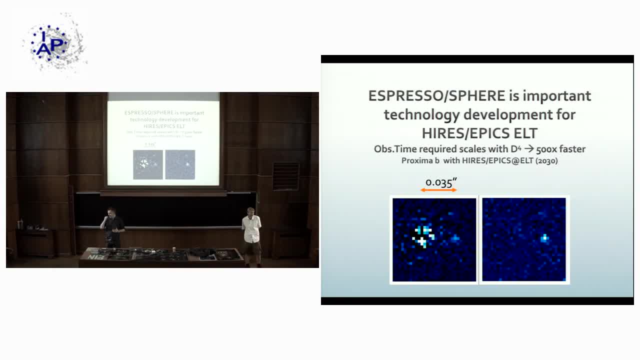 not actually do this work. A low resolution spectrum is fine and please use actually that, because you spread out your photons over a very large number of pixels. that doesn't help you observing faint targets, However, observing from the ground, using optical or even just imaging- 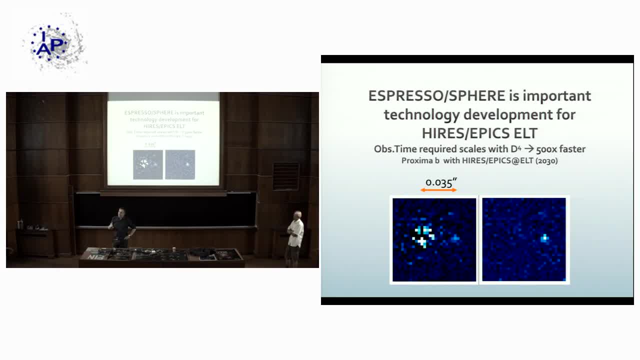 or in a filter band is very difficult because of the atmosphere. So we are looking at- if you now do not think at the direct imaging case but at the transit case. you want to see what's happening with your telescope to a star. it's. 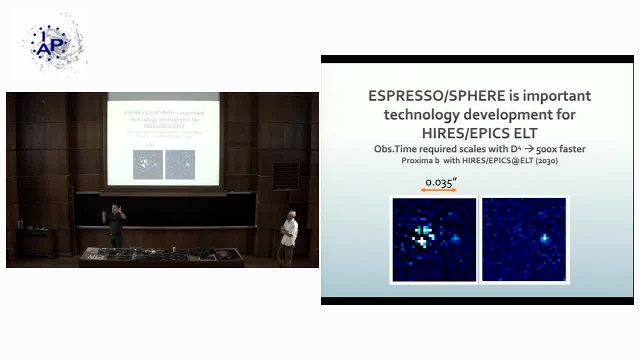 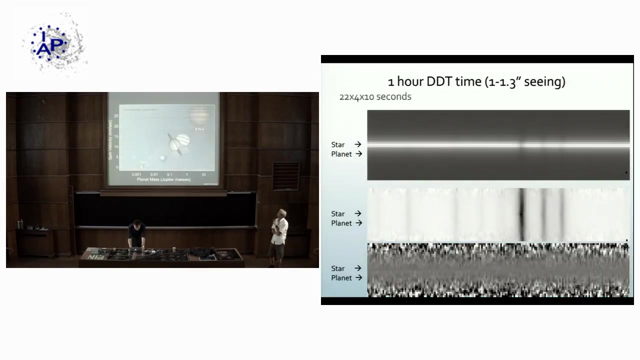 not going to do that because the actual atmosphere fluctuates at a significantly higher level. So what you can do is to have an external reference star and see the actual atmosphere and see what's going on in the atmosphere. So if you now go to 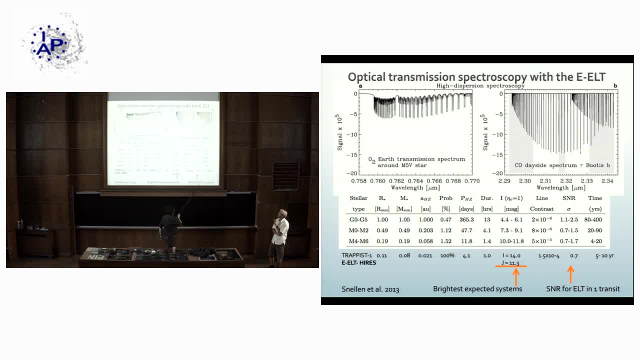 the very high spectral resolution, and maybe I can show you this. for example, with this spectrum, this spectrum, you can see that the atmosphere is changing from one wavelength to the actual length. These are all except for the atmospheric lines, Basically from 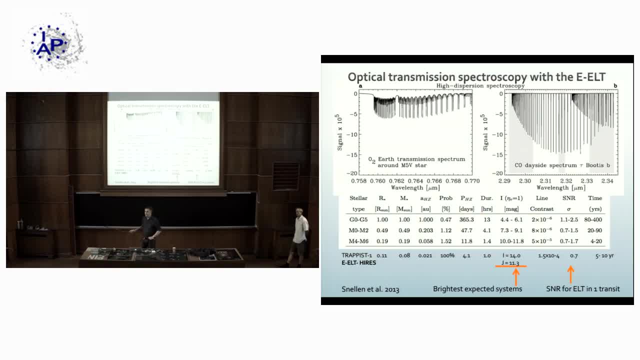 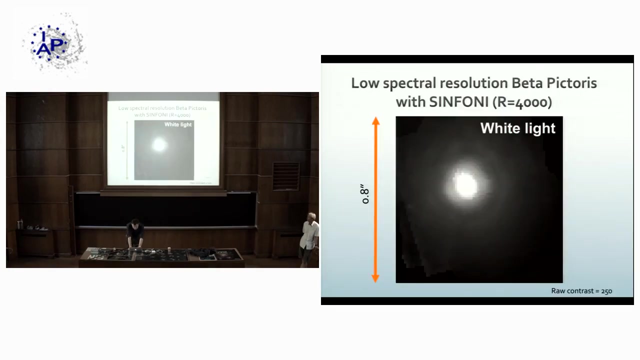 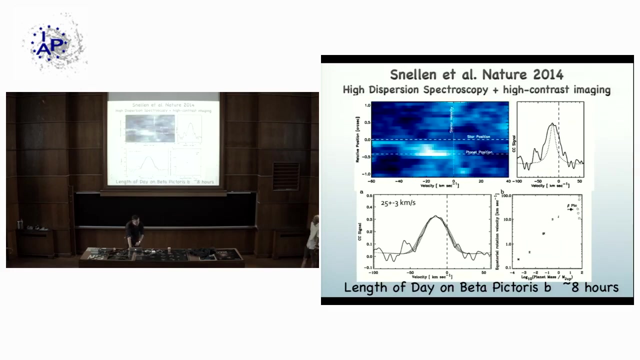 one wavelength to the next. the atmosphere is changing from one wavelength to another wavelength. So if you have a high spectral resolution spectroscopy, what typical broadening of line do you expect for these lines? Is this a typical profile? if you would have? 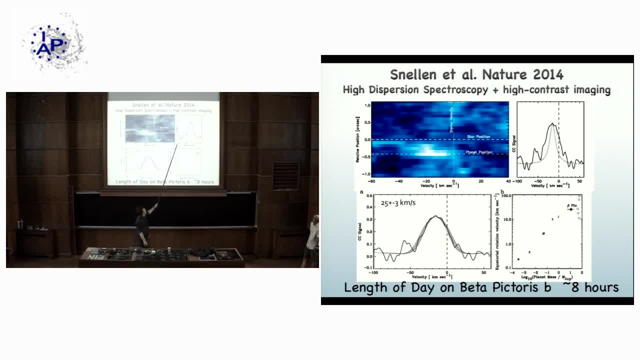 a non-rotating planet. This dashed line here is what you expect, And that is caused by the fact that, away from the atmosphere, with high pressure, That basically gives you the broadening of the line, In this case because the planet is. 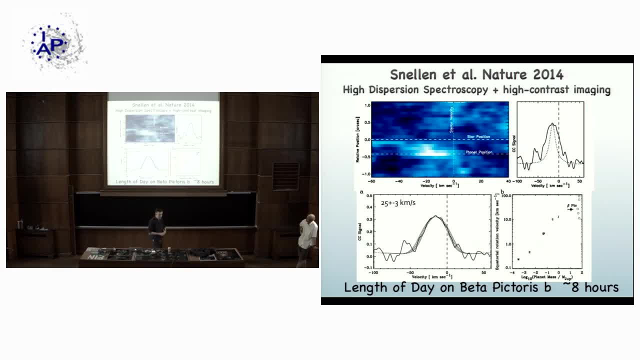 spinning that is dominating the broadening of the line. But if you would go to planets like earth or the Jupiter, which are the center of the planet, Does that sort of? Yeah, I'm just thinking now, what is causing this broadening? 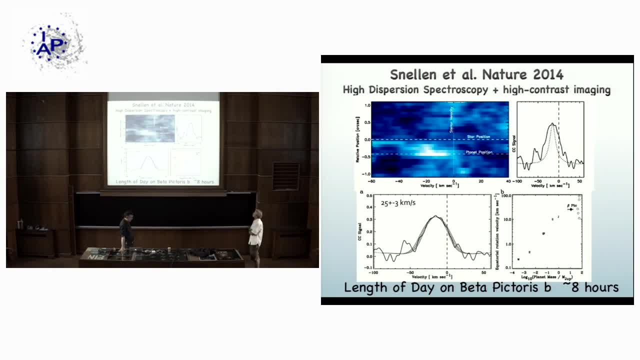 Is this collisional broadening, Matt? Probably Yeah, I'm not sure. Yeah, so we have been doing this also at lower spectral resolution, So even down to 5,000.. But then the contrast of the line become a lot. 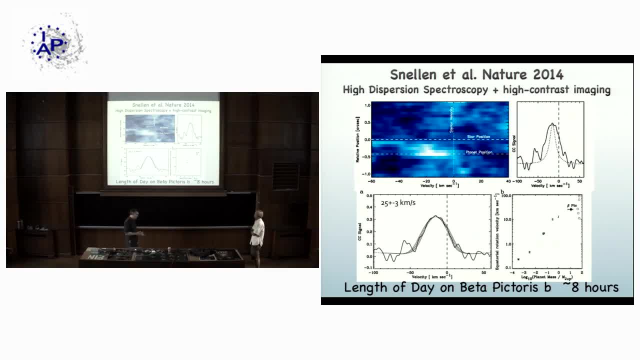 small, So it's going to become less deep, But I think that the method still actually works, although the removal of the earth's atmosphere already becomes a bit more difficult. And if you really go significantly at Keck, there is the NURSPEC. 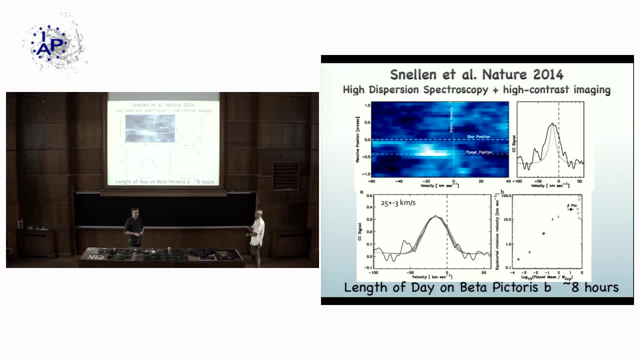 that uses a resolution of 25,000, you can already see with that that it's a lot smaller. So I think that